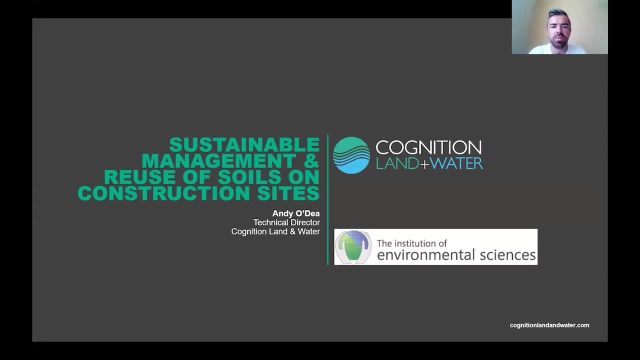 for questions at the end of the presentation. so please submit these in the Q&A option at the bottom of your screen at any point during the presentation, and I will submit these later on your behalf. Thank you for logging in today, and I'll now hand over to Andy. 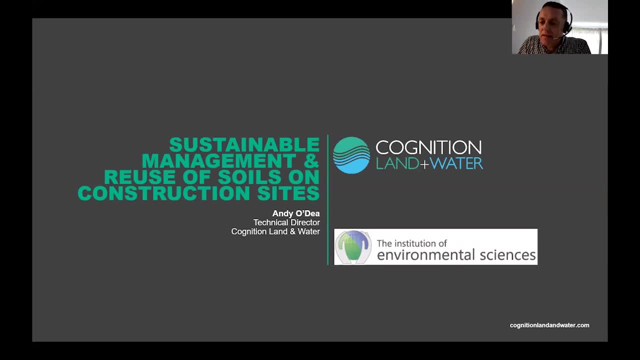 That's great. thank you very much, Derek. Good afternoon everyone, and thank you for taking time out of your day to join me on this. Despite my camera looking very gloomy, it's actually a lovely sunny day here in Reading. so, yeah, thank you for taking time to join me. As Derek said, I'm going to be talking about 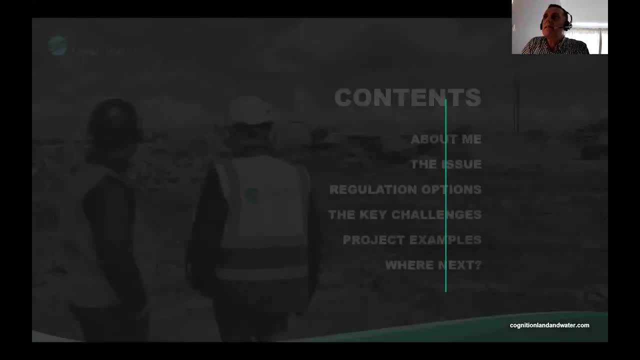 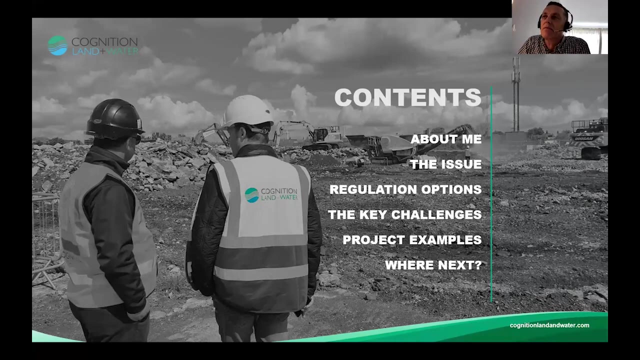 sustainable management and reuse of soils on construction sites. Some of you will know a fair bit about this subject, some of you maybe a little bit less, so a bit difficult for me to sort of pitch this at the right level, but hopefully there'll be something in it for everyone and in the Q&A at the end maybe we 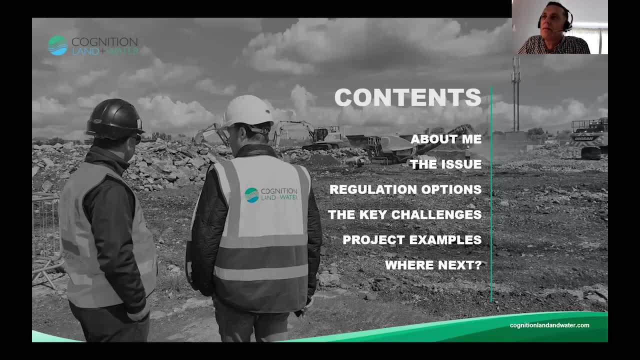 can cover some grants, some technical or more detailed queries, if you have them. So what are we going to cover in the next half hour or so? I'm going to tell you a little bit about me- I think that's important- my background and also a bit about cognition, where we 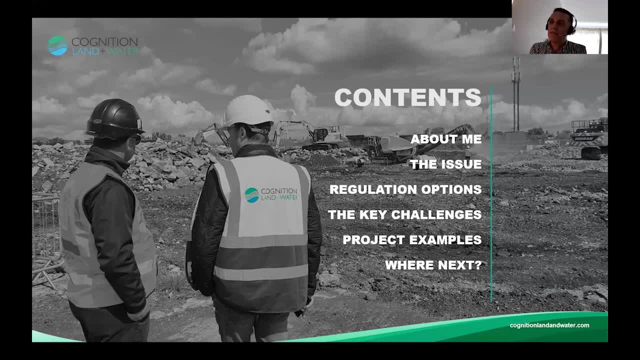 fit into this issue: The issue itself why sustainable use of soils is so critical, so important. Some of the regulation options- how do we actually regulate and how is the reuse of soils and construction sites regulated? and some of the challenges, some of the key challenges that. 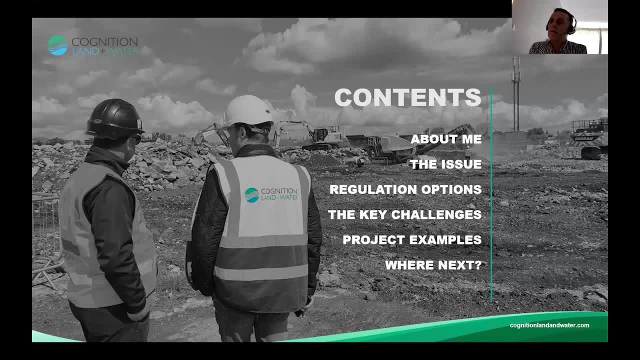 we have in that respect at the moment in our industry. I'll cover a few project examples where we have had some really good successes in terms of sustainable reuse of soils on construction sites, land development projects in the main, but also infrastructure projects and then where next. 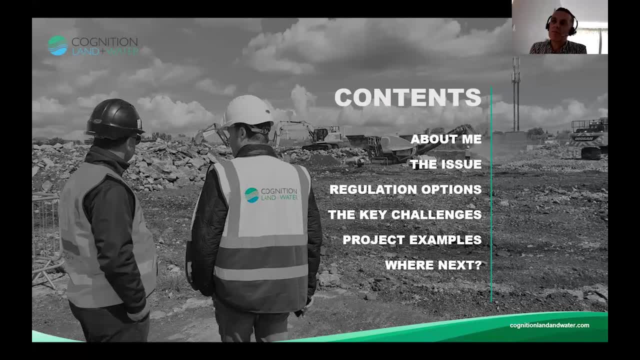 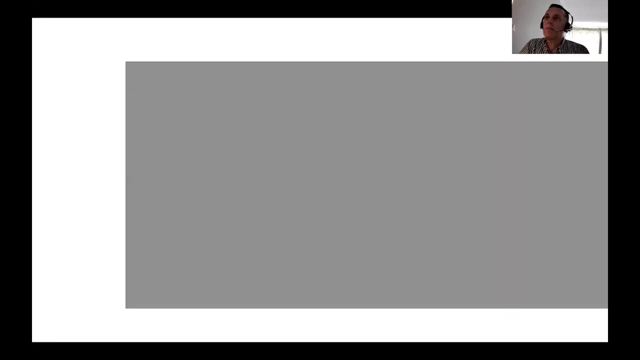 Where does the industry go? to what we have? We're sort of facing a bit of an impasse really in the industry in terms of the regulation of the reuse of construction soils. so some suggestions as to where we might go next. So a little bit about me. as Derek said, I'm Andy O'Dea, I'm a technical. 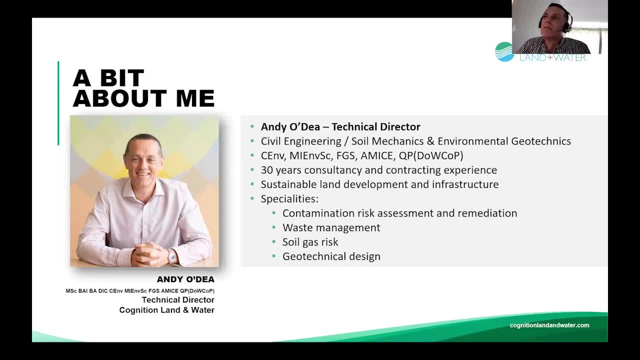 director. I'm a civil engineer by background and then moved into soil mechanics and environmental geotechnics- contaminated lands. I'm also a chartered environmentalist. I've been a member of the institution of environmental sciences for I think it's about 15-20 years now at this stage, but also, as you see, from those 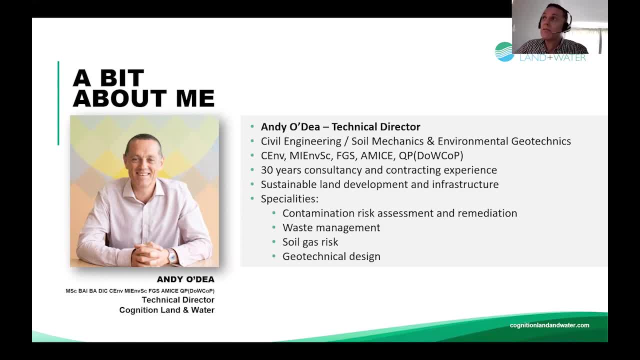 letters there on the screen. I'm also a QP for Dowcop. Now those I'll explain a little bit later on what Dowcop is and what a QP is, which is a qualified person under that scheme and why that's so important. 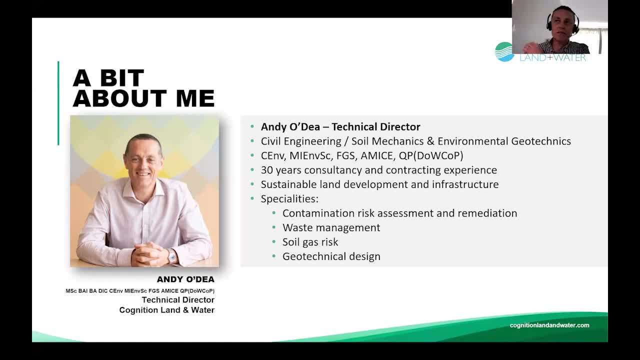 In terms of the topic, I have 30 years- more than 30 years- experience, mainly in consultancy, but moved across to contracting three and a half or so years ago. so I suppose I can give you a perspective from the design and consultancy side of things, as well as the contracting side of things. 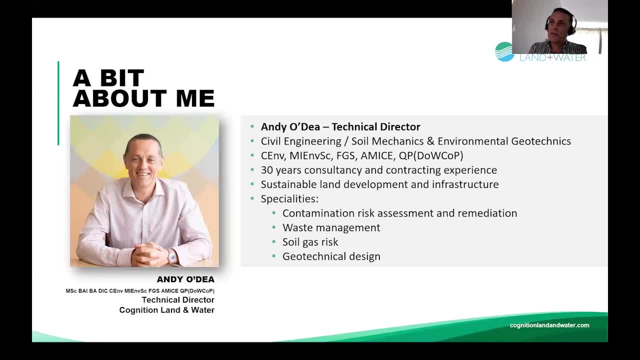 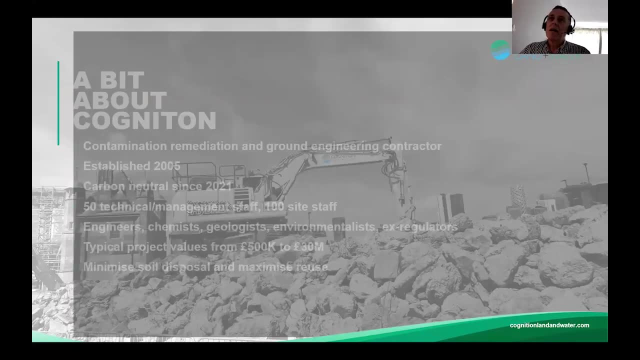 and almost all of my work over those 30 years has been on sustainable land development and infrastructure projects I specialised in. I specialise in contaminated land risk assessments and remediation, waste management, soil gas risk and geotechnical design, And a little bit about cognition. as I said, I worked for Cognition, Land and Water. this 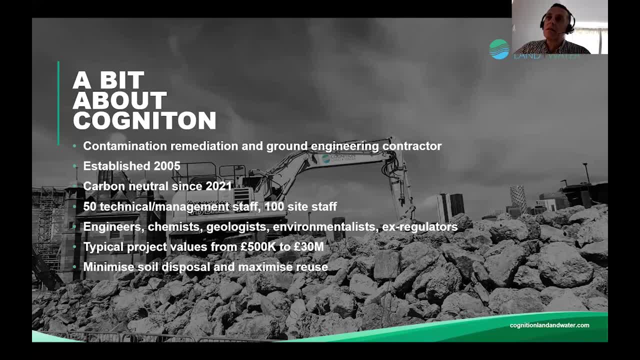 isn't a sales pitch for us as a contractor, but I think it is important that you understand our background and where we come from and why I suppose I'm giving this, this talk today, to raise awareness. We are a contamination remediation and ground engineering contractor. we've been 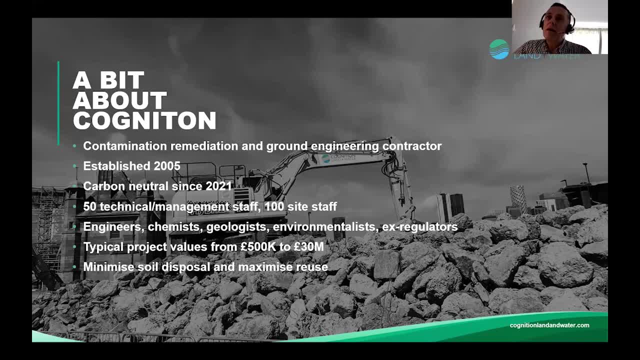 around for about 20 years years or so. uh, we became carbon neutral as a company um over two years ago now, uh, which is we're very proud of that and it's very important to us, and one of the biggest ways that we actually uh achieve that is is in the uh in the work we do in terms of uh reuse of soils, minimizing uh. 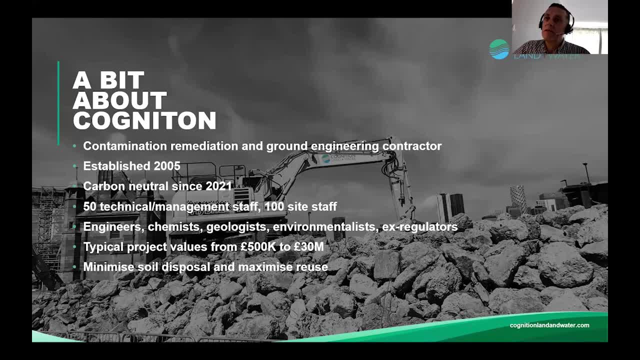 disposal to landfill. we have about 50 or so technical management staff and about another hundred or so side staff um and we're of a broad range of uh of skills and experiences within within the company: engineers, chemists, geologists, environmentalists and, very importantly uh, several ex-regulators as well- excuse me, people who've um who've worked many years in the uh in. 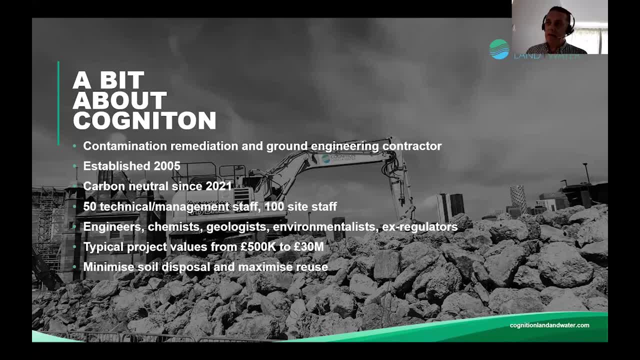 the environment agency and local authority and they give us that sort of um perspective but that we bring to our work typical projects that range from about half a million to 30 million, and minimizing soil disposal and maximizing reuse on construction sites is, in my mind, is everything. 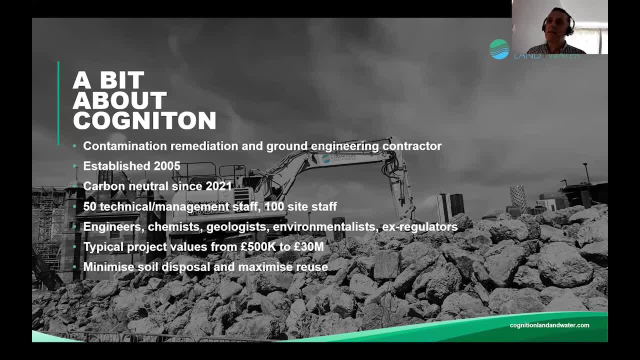 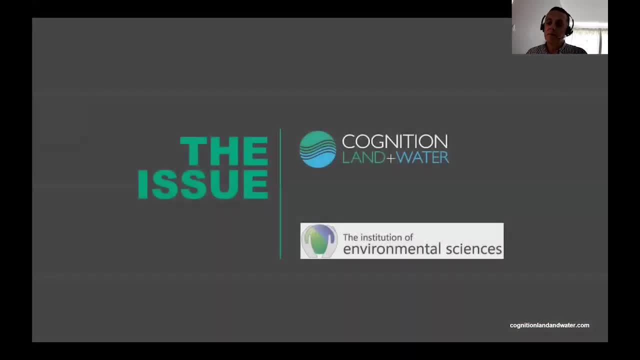 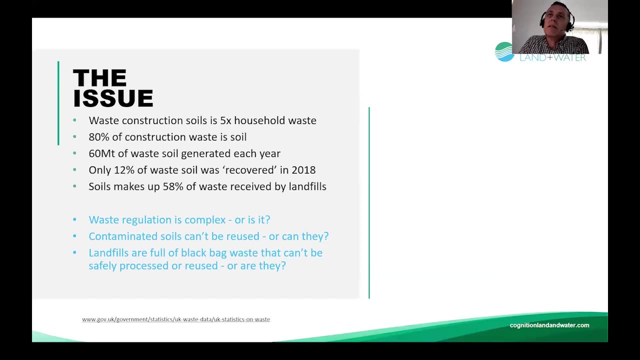 that we do. that's where we have the greatest impact by far in the work that we do um avoiding disposal of soils and filling up landfills unnecessarily. so what is the issue? um, well, it is a huge issue in our, in our industry, waste construction soils are equivalent to five time. 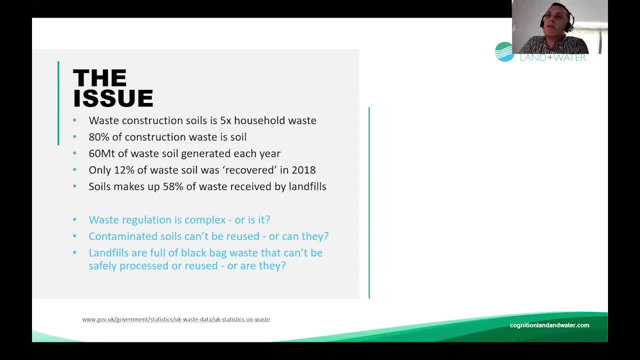 uh five times um domestic waste that's generated in the uk. in an average year, uh eighty percent of construction soil. uh construction waste is soil. uh soil is a hugely valuable resource. um we really don't want to be um creating uh a waste from that material and and disposing of it uh 60 million tons of. 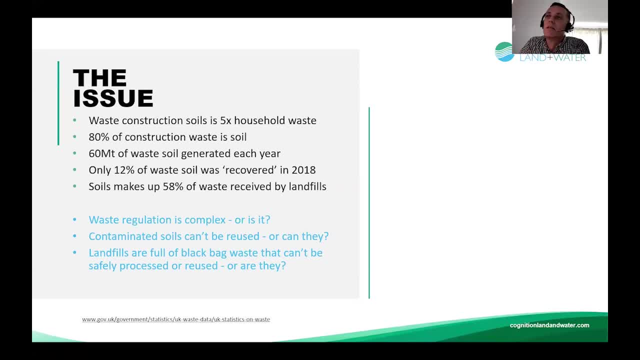 waste or uh waste soil are generated each year in uk. these are these- sorry, i should say that these are- are um government statistics from 2018.. the most important year in the year 2018.. the most recent um uh data available and, shockingly, only 12 percent of waste soil was what's officially 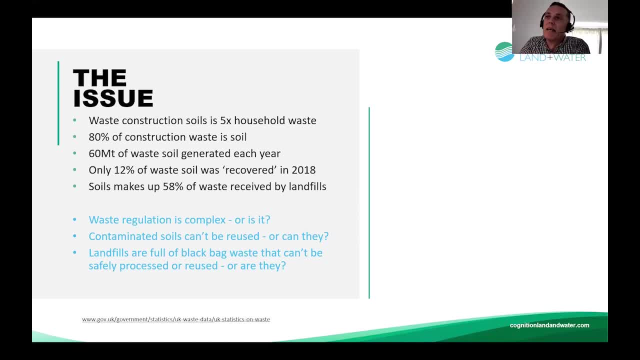 called recovered in 2018.. uh, i personally i think we should be ashamed of ourselves and embarrassed as an industry that that this is what we're doing. um, soils make up 58 of the waste that's received by landfills. um, and these sort of statistics are really terrible. we we need to be doing a lot. 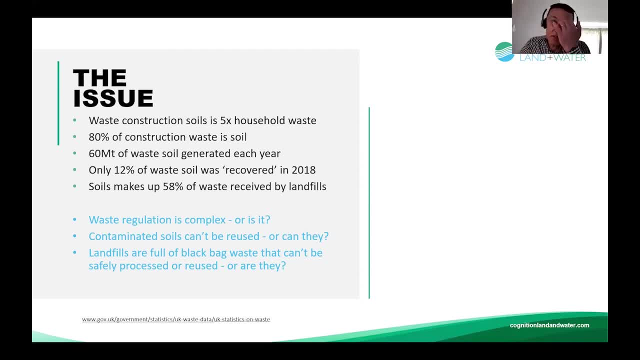 better. but uh, hopefully you'll see uh in the next couple of weeks we're going to be able to do a lot better. but uh, hopefully you'll see uh in the next couple of weeks we're going to be able to do a lot later on in the presentation- that there are lots of hurdles in the way. 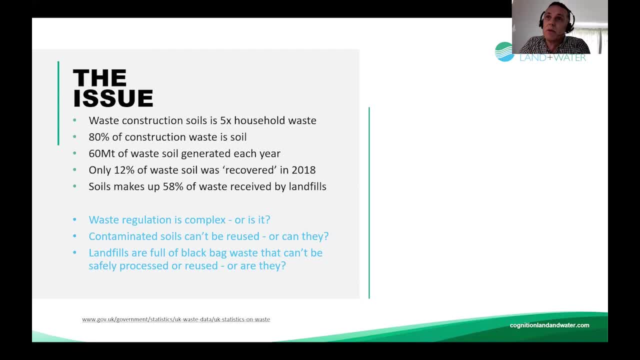 of uh, of achieving veterans in terms of those, those numbers, um. some would say that waste regulation is is complex, time consuming. time consuming, yes, it is, um, there's no doubt about that. but it's not insurmountable, it's not beyond the way to man for us to um, to, to get over this uh. 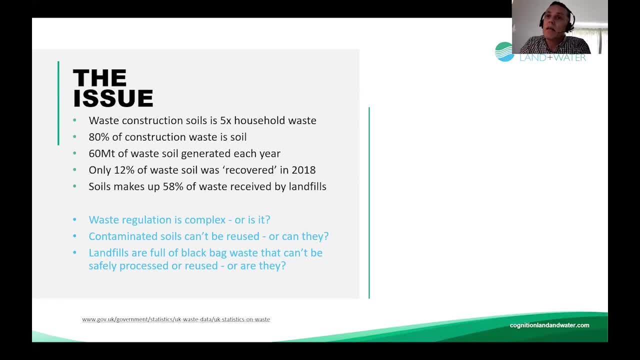 this issue um the law and regulations. uh, some say the contaminated soils can't be reused on sites. um, i disagree completely and we've got lots and lots of examples where contaminators, soils, can be remediated, cleaned up, made suitable for use and reused on construction sites where they present. 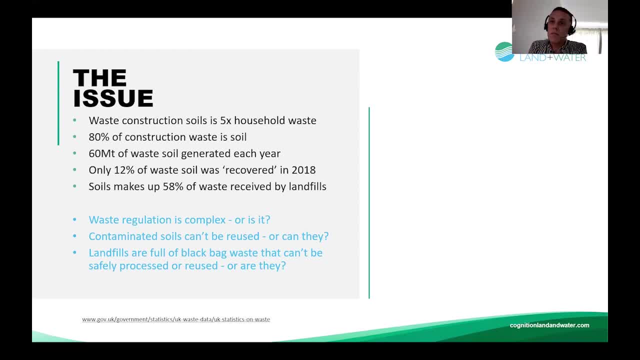 no risk to the environment or future users, and some say that lambs fills are full of black bag waste that can't be safely processed or reused again. i have lots of experience, we have lots of experience on on regenerating, remediating um uh old landfill sites and bringing them. 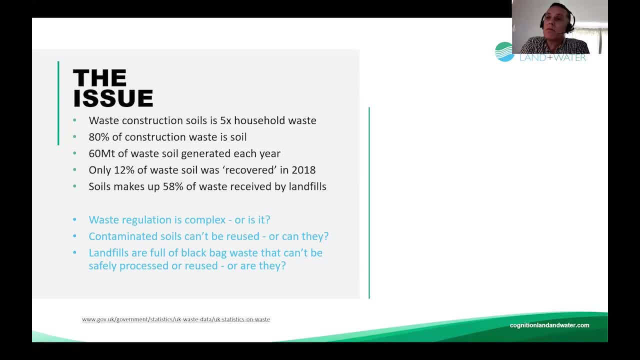 back into beneficial use and that is absolutely not the case in the most, in most of those, on most of those sites, 80 to 90 of the material that's in those landfills is soil that can be recovered, reused on sites. so let's do some debunking, as i've said. um. so what i suppose? um, you may ask. 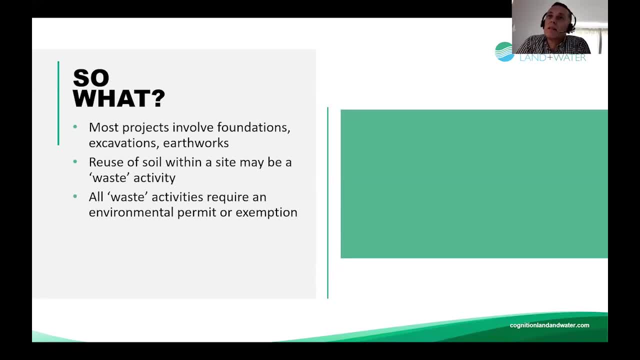 yourself. why is this important? um, most of the projects that uh that you, um and i maybe get involved in uh involve foundations, earthworks, excavations and generating soil. you may not know, but reusing that soil with inner side may actually be a waste activity if you don't. 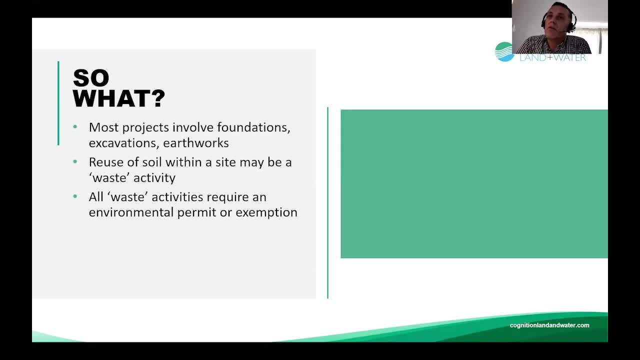 control, manage, record that process. you may unwittingly be creating a waste and depositing your waste and there are implications to that. um that that i'll talk about in a bit. and all waste activities either require an environmental permit or an exemption from an environmental permit. so the result of this is that in the uk, thousands 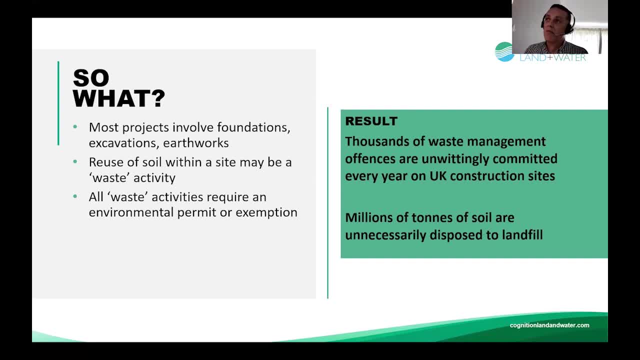 of waste management. offenses are unwittingly committed every year on uk construction sites and millions and millions of tons of soil are unnecessarily disposed of to landfill. i have lots of examples. uh, those of us in the contracting side of the business, of the industry, i can give you plenty of examples of where that's the case, uh, where we really should be reusing those soils on. 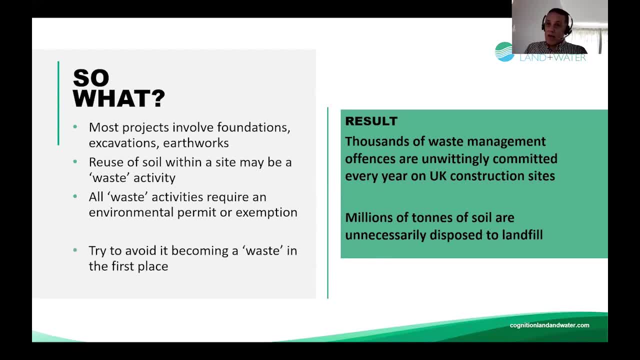 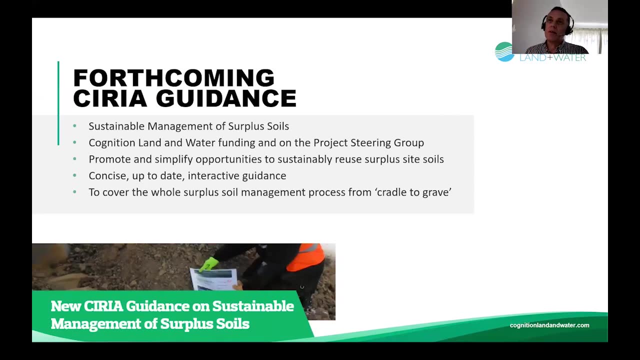 site and not putting them in landfills, and the easiest way and the best way to um to to avoid that is really to avoid it becoming defined as a waste in the first place again. i'll explain in a minute why that, uh, how we can do that. first of all, though, i'm gonna um give a a shameless 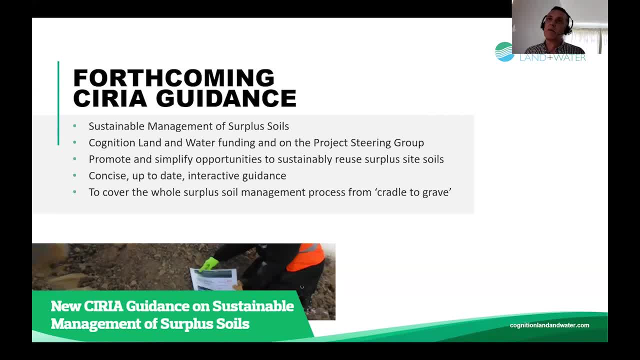 plug for uh for an upcoming uh guidance document from syria. uh, some of you should be familiar with syria, which is a construction industry research and information association. um, and i've been involved in this on the project steering group for this, this guidance document. uh, cognition have also funded it, um, because we see it as being extremely important. 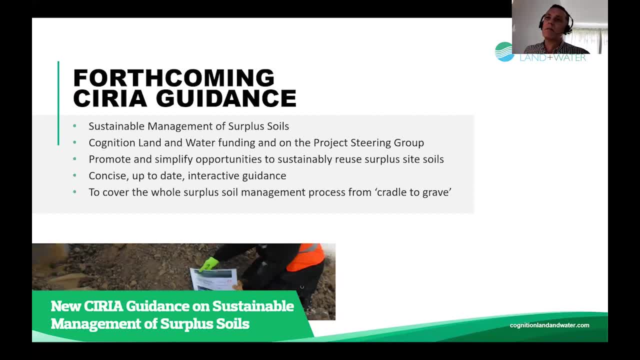 and really this is a a a way of promoting um and simplifying opportunities to um to reuse surface soils on site. the idea is that it's it's concise but comprehensive, up-to-date and interactive guidance that explains the whole process of soil management, from cradle to grade. so keep an eye out for that. it's um, it's, it'll be coming, it'll be published. 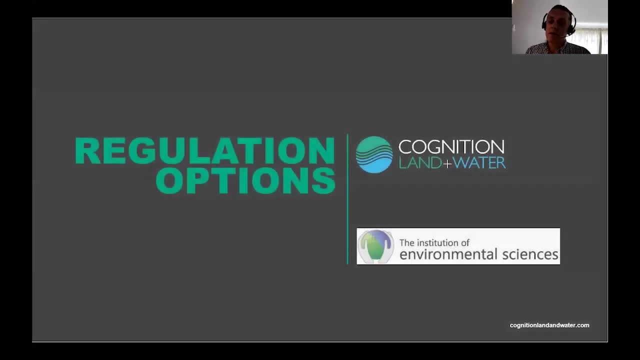 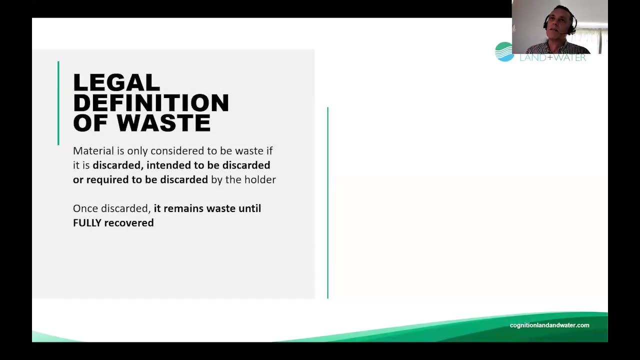 within the next few months. so some of the regulation options. before we go into that, it's important that you understand what is a waste, and there is a legal definition of a waste. lots of you will have heard of this before, i'm sure, and really discard- discarded is the important word here. so a material is only considered a waste if it's discarded. if you 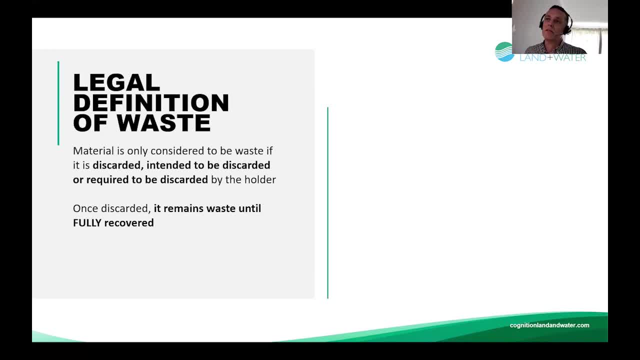 intend to discard it, or if you're required to discard it and that's enshrined in in law? um, but once a a material is is discarded and it becomes a waste, it remains a waste until it's fully recovered and there are only certain ways in which that? um that material, that 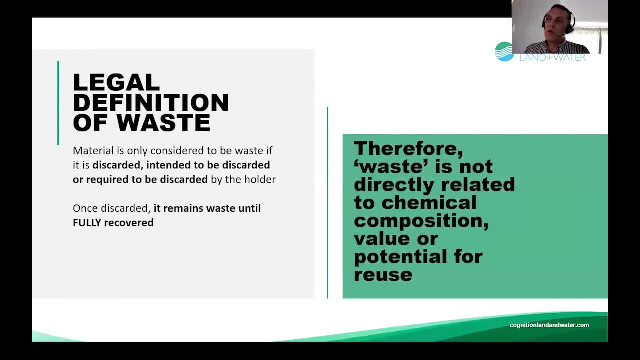 soil can be recovered. it's important to know, therefore, that waste is not related to its chemical composition. a material can be contaminated, and it can be contaminated in certain situations. it can still be suitable for use on a site if used in in a particular way, or it can be remediated. 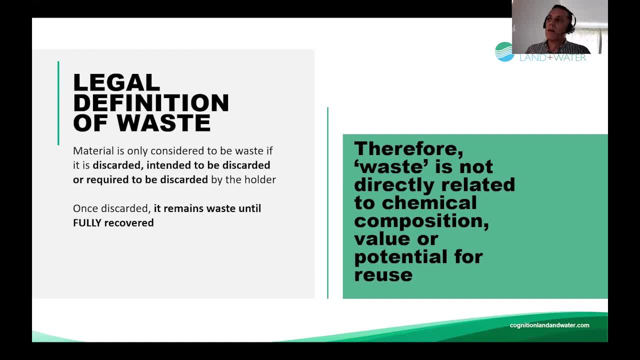 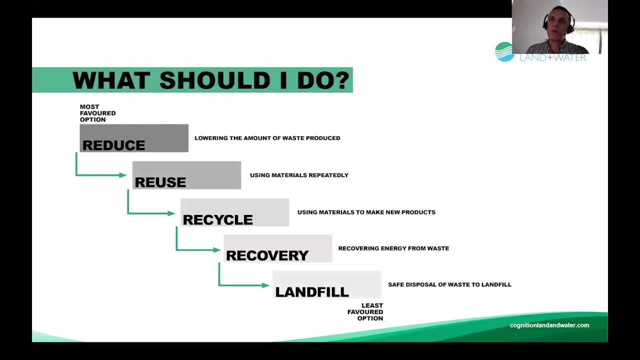 and treated to make it suitable for use. um, it's not necessarily a waste if it's contaminated, or even if it has a value to you. if you're still discarding it, then it still could be a waste. so what should you do? um, hopefully you'll all be familiar with. 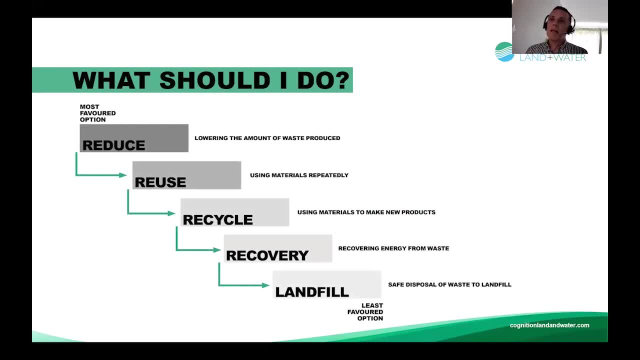 this the waste hierarchy. what we really need to be doing is um, in terms of the management of of soils and construction sites on the in the way in the waste hierarchy, so reducing the amount of uh of waste that we generate. and if we can't reduce it, then 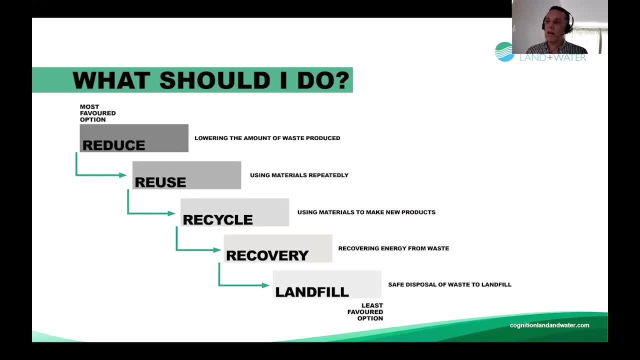 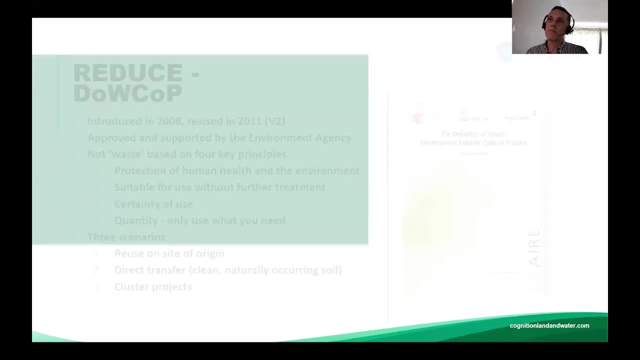 we reuse it, recycle it, recover it and so on. and the last option absolutely should be um landfill. that's the least favorite option, sending soils to landfill. so i'm going to run through. so just to go back, i'm going to run through that sequence um reduce, reuse, recycle, recovery. 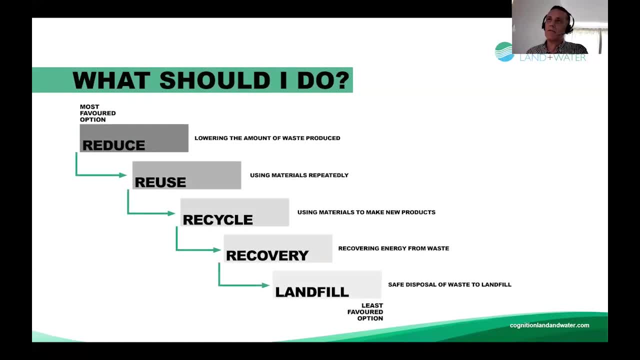 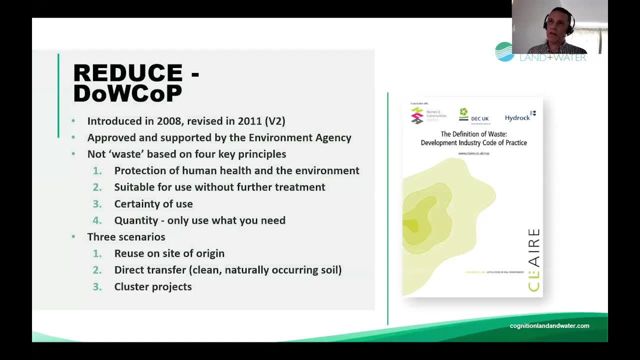 cover and dispose in the following series of slides and give you examples of how that process is regulated. The top one and the one that I think is really the best tool that we have in the industry at the moment for reusing soils on site and a tool that avoids a soil being defined or 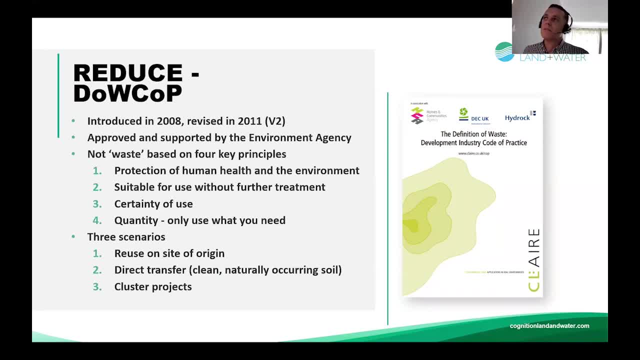 classified as a waste in the first place is something called the DAUCO. This is the definition of waste industry code of practice. It was introduced in 2008,, so it's been around for about 15 years or so. It has been revised. 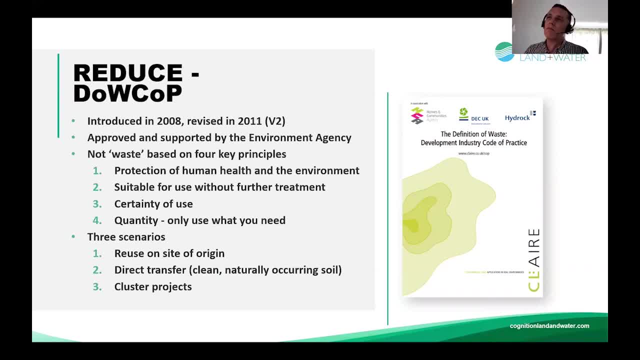 There's a new version. that's imminent. that's been with the Environment Agency for quite a while. We're waiting with bated breath for that to come through version three. Originally, this document and this process was approved and supported by the Environment Agency. 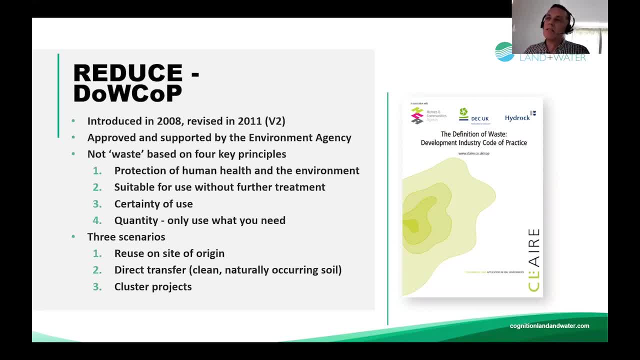 I'm afraid to say that the Environment Agency in some respects seem to be having sort of co-feet in terms of the use of the guide and things have changed recently in terms of the acceptability of using this DAUCO process in certain situations, which is unfortunate. 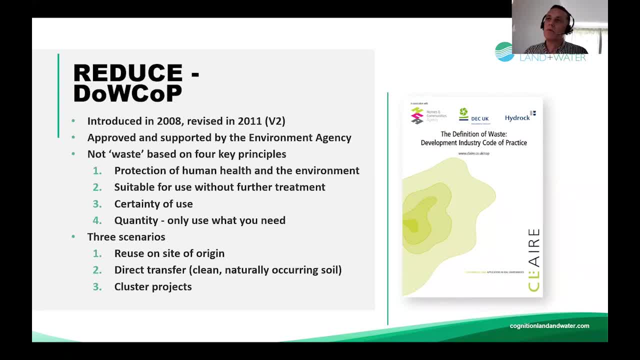 I think, because, as I said, I think it's the best tool we have By applying the process. By applying the process in the DAUCO, you can soil does not become a waste on a construction site if it achieves these four key principles. 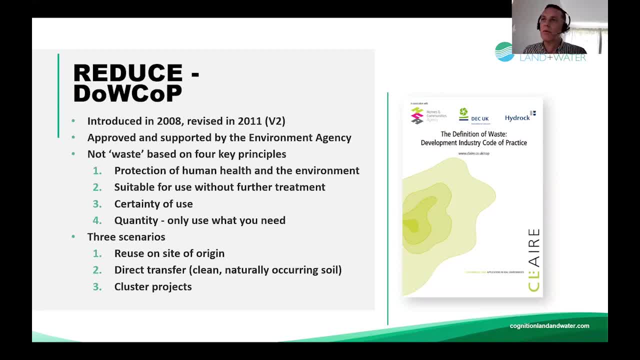 First one is that it needs to be protective of human health and the environment, and everyone would agree with that. that's fine. It needs to be suitable for use without further treatment. Again, that's fine. if the material is suitable, then it can be reused. 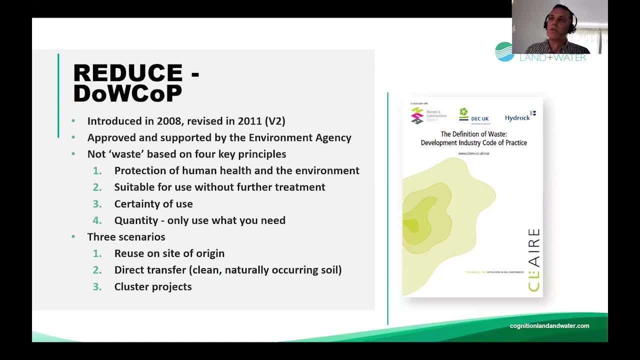 It can be treated under, let's say, a mobile plant permit before it's reused, And those two in combination- the mobile plant permit and the DAUCO- could allow for a material to be reused on the site. There also has to be certainty of use. 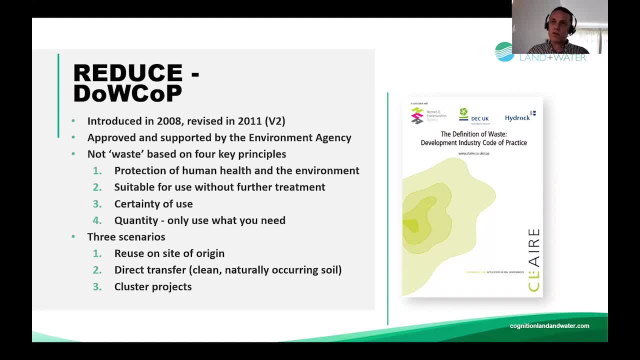 It can't be just the mere possibility that a soil is reused. So sticking something in a stockpile and leaving it there for a couple of years is not acceptable under DAUCO And I don't think it should be really. But usually we tick that box by under if there's a planning condition or something. 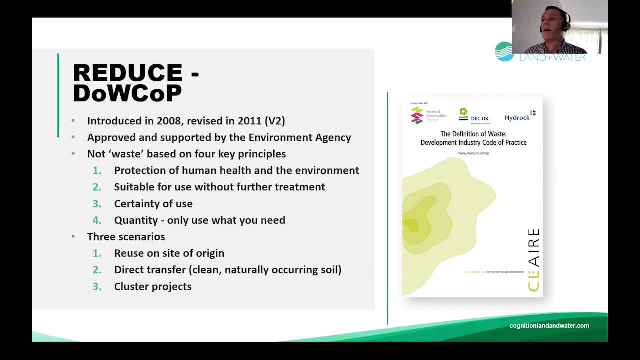 That's fine. That's fine, That's fine. But certainly it's a good idea to have a planning consent on the site And that demonstrates that there is certainty of use if that soil is part of a planning process And, importantly, the quantity is important. 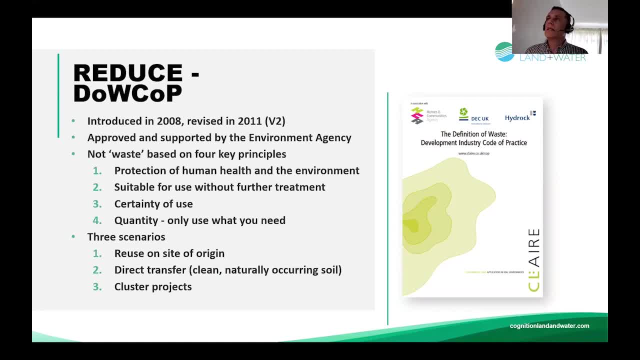 You can only use what you need to use on the site. So you can't create, for example, a large environmental bund if that's not specified as part of the design of the works. So you can't be discarding or getting rid of it. 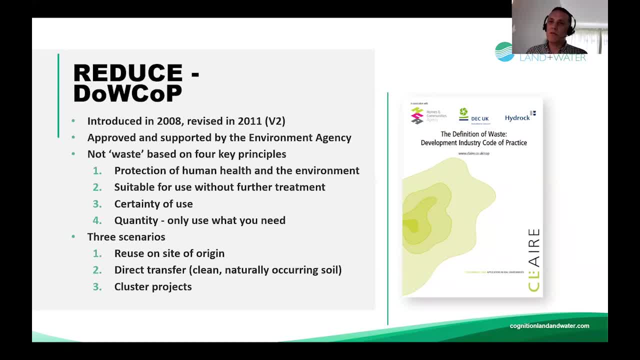 Or it's like: what's wrong with this rid of material on a site? you have to use only what you need to use and under the dark up. there are three different scenarios. so you can reuse materials on the site of origin. so within one development site, you can take material from one part of the site to the other, let's say a foundation. 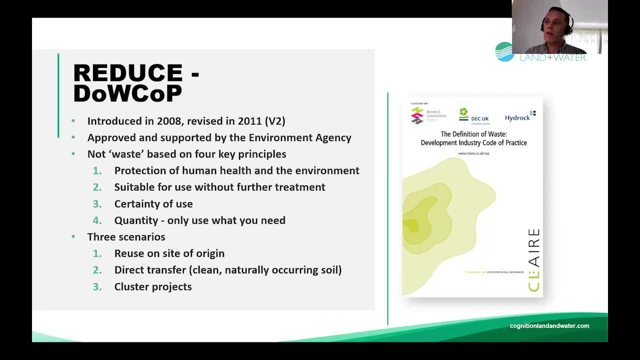 excavation and reuse it somewhere else on the site and that can be made ground or it can be natural soils on that site. you can transfer materials- soils- between sites, which again is extremely helpful, but in that instance you can only transfer clean, naturally occurring soil under the dark up. you can't transfer made ground between one site and another. to do that formally you would. 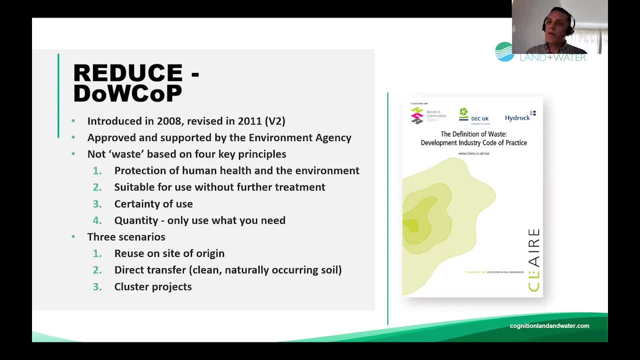 need an environmental permit or an exemption. and then there's a third scenario, which is a cluster project, or a hub and cluster as it's sometimes called. that's where you have a hub site, a central site that accepts or takes in site soils from a donor's, a number of donor sites, and that can be. 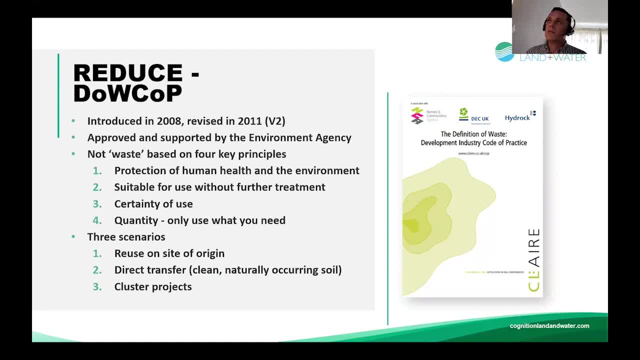 made ground or natural soils, then that material is processed, tested, sampled, make sure that it's suitable for use and then it can be exported back to either the original sites or to receiving sites, once it's confirmed that it's suitable. again, unfortunately, the cluster projects is something. 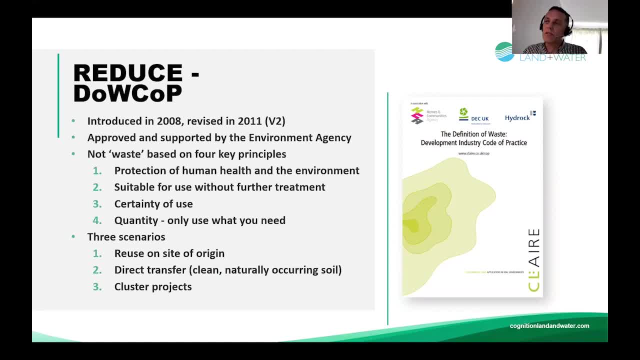 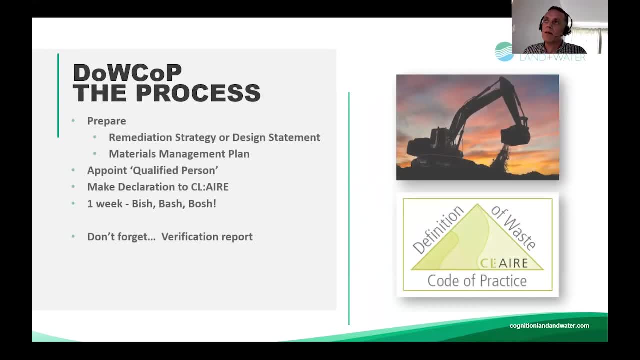 the environment agency is scrutinizing extremely rigorously at the moment and there seems to be a an issue with accepting cluster projects in many cases. so what's the process under dad cop? it's? it's very straightforward, which is, i suppose, one of its um, it's its attractions, um. you produce a remediation strategy, or um, as you would normally. 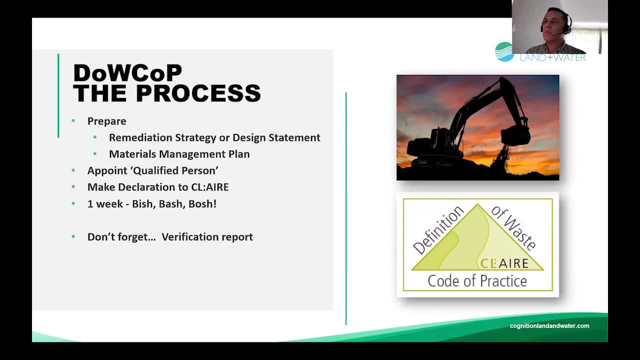 i suppose on the side, or if there isn't a remediation strategy and it's a simple project, then you can produce a design statement, which is a very simple statement, to say that the material, but the composition of the material, and um to say that it's suitable for use. you could pick. 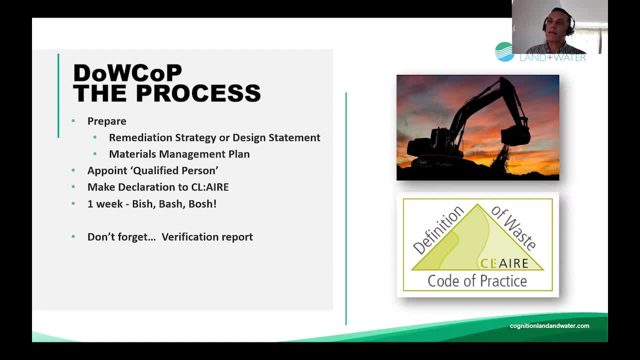 the key document for the dark up is a material management plan and that outlines the parties involved, um the nature of the development, the sources of the soils, the where they're going to, um how you're going to track that and record it. and all that material, all that information, goes together into a single document, a verification. 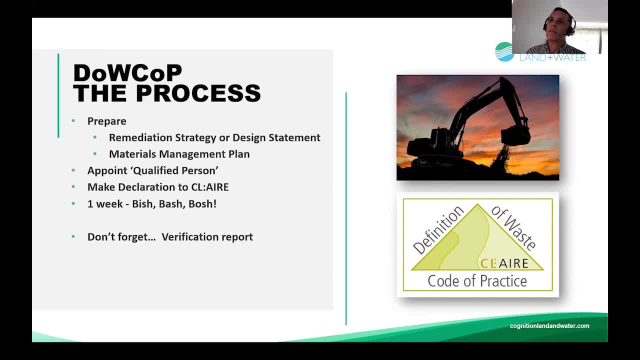 report which you produce at the very end of the project and and submit to um, to claire, um, but before that, once you've produced the materials management plan, you then appoint a qualified person and um, that's what i said i was earlier on at qp: um, that person has to be completely independent of the project. um, they don't have to be independent. 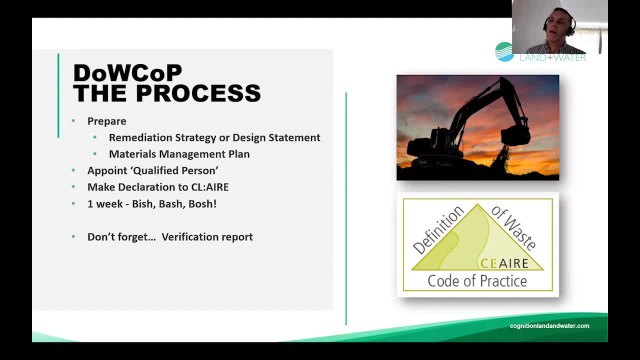 of the company. they can be within the company but they can't be involved in the project. and that person um has a certain level of understanding, has gone through a test, an exam process with with claire, to demonstrate that they understand the application of dow cov. they 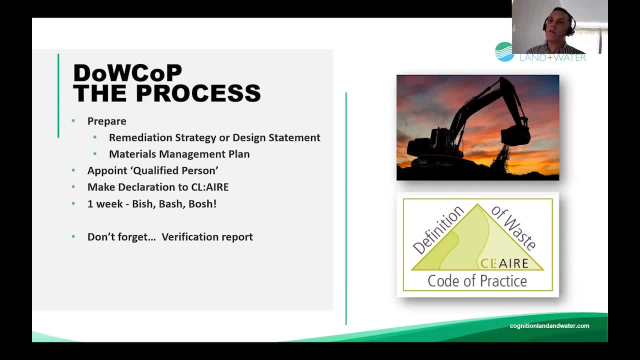 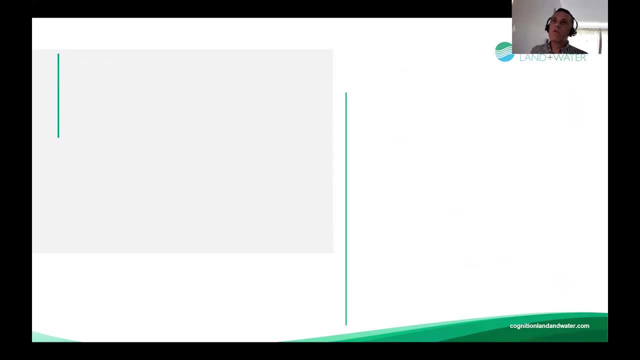 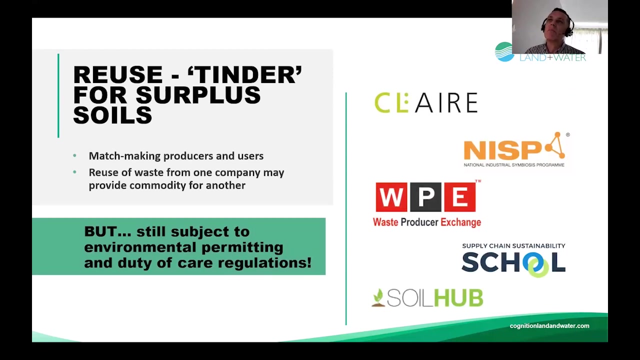 view all the information they submit, the declaration to claire, which is the organization that manages the process, um, and all of this can be done in a week or so. bish bash bosh, as i said, very straightforward, very, very easy. moving on to reuse: um, uh, there is a another option where materials can be, uh, moved between sites. 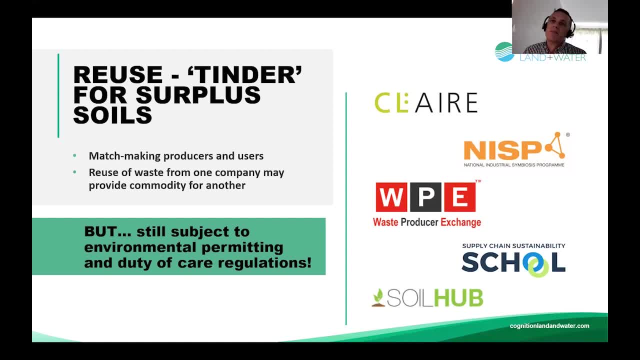 i'll call this tinder for surplus soils and basically it is. that's what it is. it's a match making, making um- process, where donor sites are connected to receiving sites and and those soils then don't necessarily become a waste and they can be transferred between sites. but you need to be careful because there are 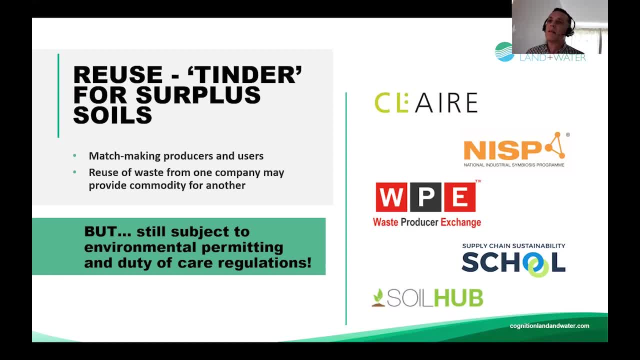 certain instances where they may become a waste and an environmental permit is required, certainly, duty of care regulations would would apply, and there are several different organizations that manage these um, these registers of donor and receiving sites. claire's is the, is the largest one um their register of sites, but then the soil hub as well, which, uh, which is launched. 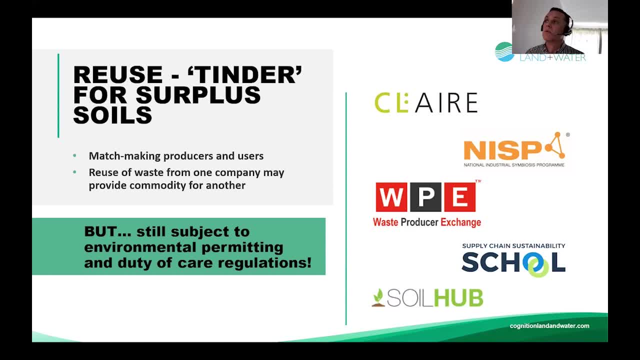 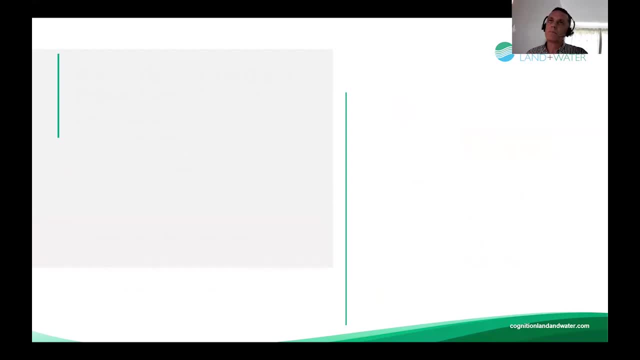 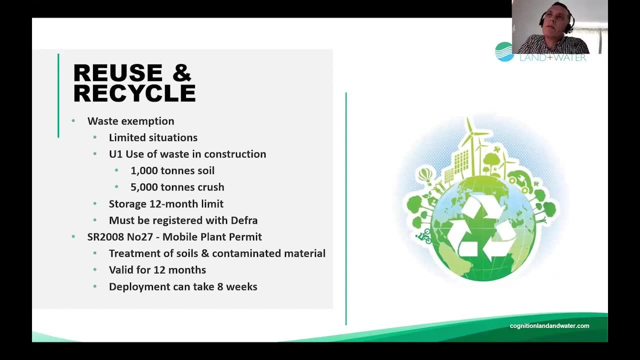 quite recently. uh, the supply chain sustainability school has one as well, and there were a number in the past- nisp and wpe- which i'm not sure they operate anymore. moving on to recycling, we're going down the, uh, the the waste hierarchy now, um, in terms of about sort of going back to reuse slightly, um, 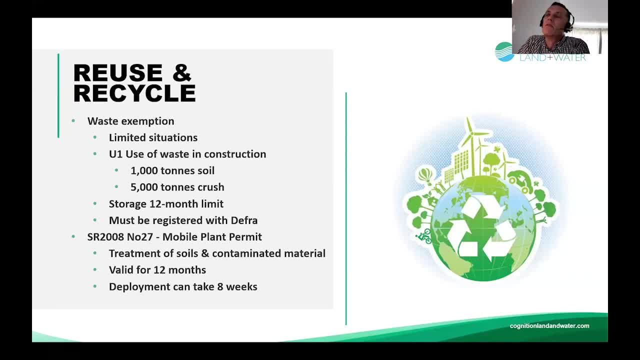 you can also, if you, if you don't have to, if you don't want to get an environmental permit, there are, there is an option to get a waste exemption, exemption from environmental permit. those are very limited uh circumstances, uh, one example is u1, which is the use of waste in construction. 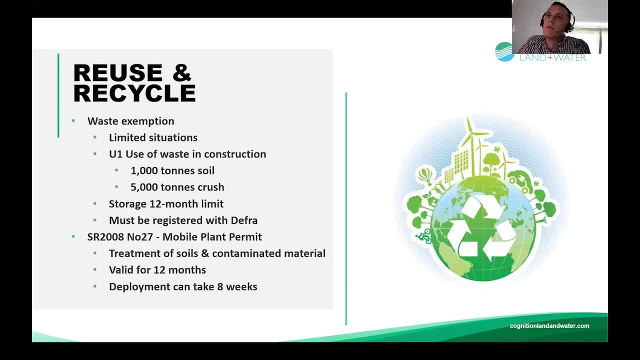 it's limited in terms of how much soil you can use um a thousand tons or five thousand tons of crush, say six f2 uh. it's limited in terms of how long if you store a material on site and that exemption must be registered with uh, with defra. in terms of recycling, um we can use a mobile plant permit for. 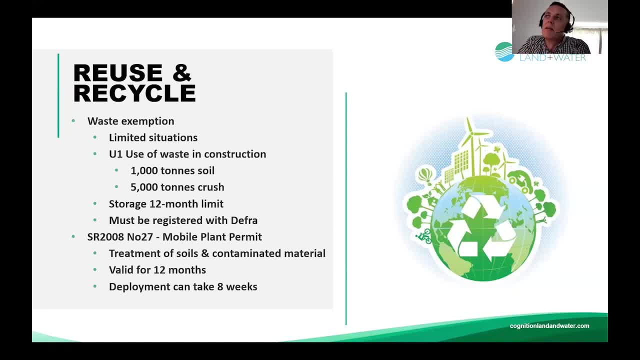 treating soils or contaminating material on site and making them suitable for for use. um cognition operates a mobile plant permit. that is, that's a standard rules permit and it's it's deployed on every uh. it's specifically deployed on on every individual site. you go through a 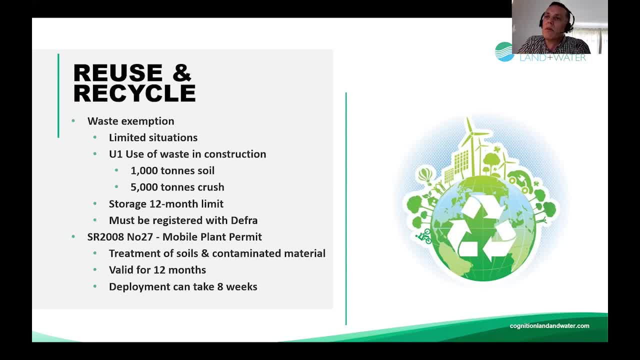 process of of demonstrating that you have full control of uh, of any potential environmental impacts. um, and that's. that permit is then valid for 12 months from the date you start the works. worth noting that the the deployment can take eight weeks or even 12 weeks, sometimes in that. 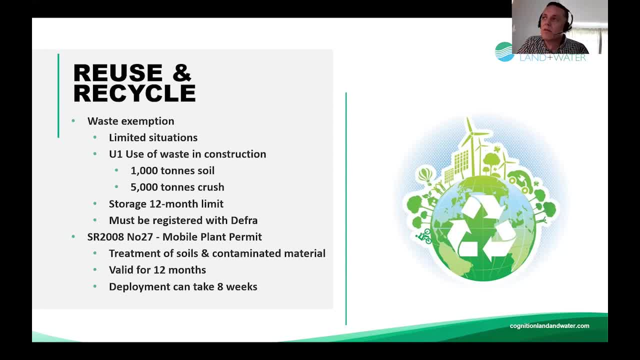 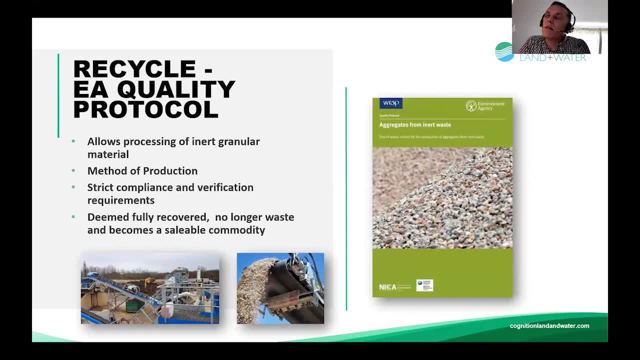 so you need to plan and allow for that as part of your your works program. recycling- this is a really good example of of recycling of construction arisings. it's. it's now called the environmental equality protocol it was. some people may know it by the its former name, the rap protocol. uh, and this one? there are a number of them, but this one relates to 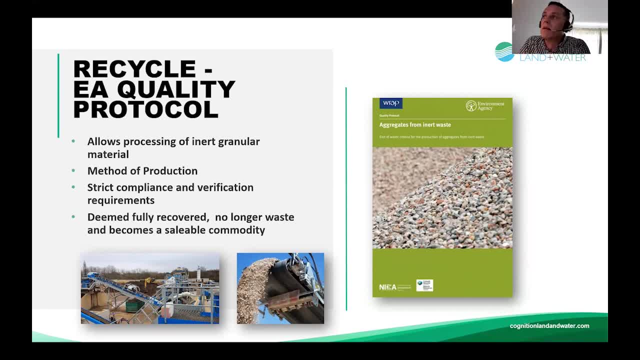 aggregates from inert waste. the best example really is um is uh production of 6f2 or crush from from demolition material, concrete crush or brick um and, as i said there, it allows the processing of an inner granular material, only granular film. um you, you, you need to produce or or prepare a method of production which is uh uh outlines. 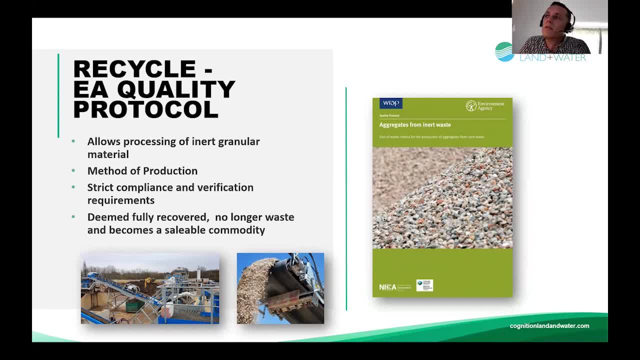 strict compliance and verification requirements to demonstrate that the material is what it should be, um. and then, once it's gone through that process and you've you've done all your verification and all your compliance, then that material is no longer a waste. it was originally. it's no longer a waste now it's a commodity, it's a product and it can be sold from the site. 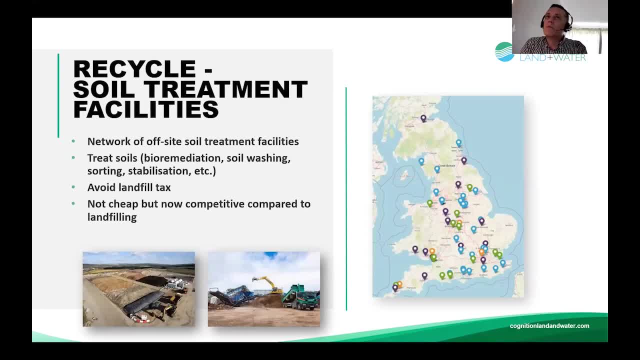 but uh continue with the process. uh, you starts to get into the materials, where the material goes and which material reaches to the site, and and which material reaches to the site after production. uh, and the, the years, that that's what the nature studies uh project, what HK would to be like. uh, then, and for that, 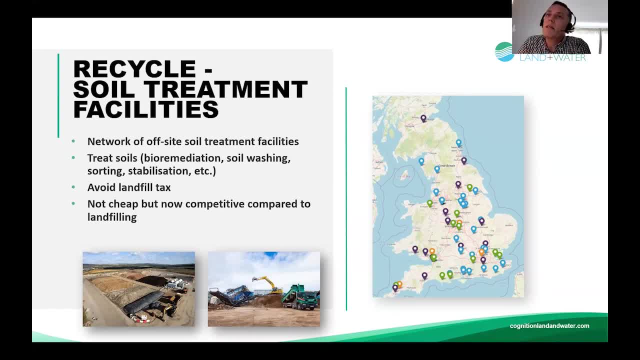 day, but you'll get it very quickly. you just you'll have to dying that bent fill to fill it simply put so much, a lot of US dollars into the um, the, the location of the facility. it's has a lot of tactical infrastructure and infrastructure. that's social things. 데jah oleapalgDe câannes. 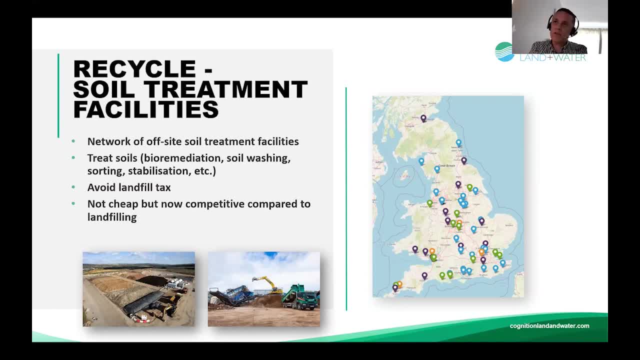 other areas, uh roughshod solar treatment facilities, soil washing or bioremediation would be for hydrocarbon soil washing, for heavy metals sorting and processing, cement stabilization or line stabilization to lock in contaminants. The great benefit of this is that, even though they're not cheap, they are competitive when 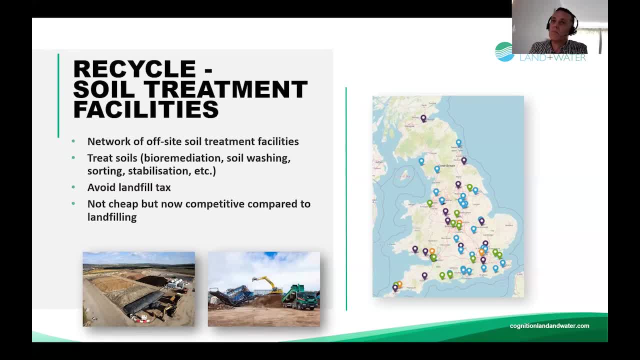 compared to landfilling, And the reason for this is that you don't pay landfill tax when you send a material to a soil-treating facility. Later on, and I think in the next few slides down, I'll explain why landfill taxes is such an important factor. 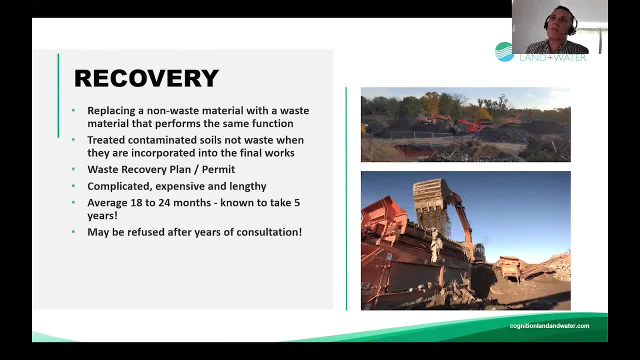 And this is the one that we are really struggling with in the industry at the moment, and this is recovery. So this is where you're looking to replace a non-waste material, such as a virgin gravel from a quarry, with a waste material that performs the same function Once the material 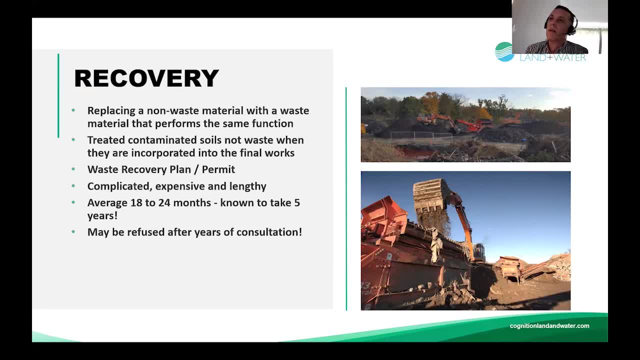 is replaced, it's a waste material. Once the material is replaced, it's a waste material. Once the material is replaced, it's a waste material. Once the material is treated, the contaminated soils are treated. they're not waste when they're then incorporated in the 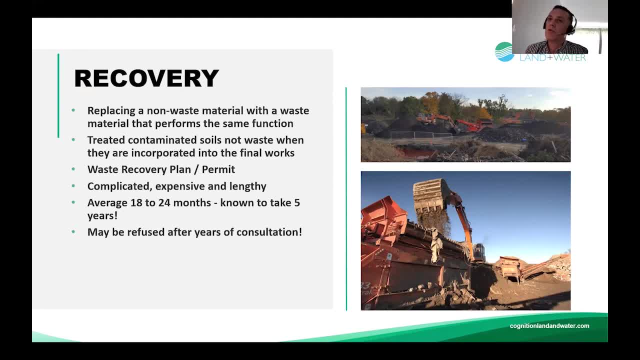 final works. So you go through this process: produce a waste recovery plan, get your waste, your deposit for recovery, environmental permit and then, once the works are completed, the soils, the recovered soils, are recovered and they are no longer waste. However, the problem is: 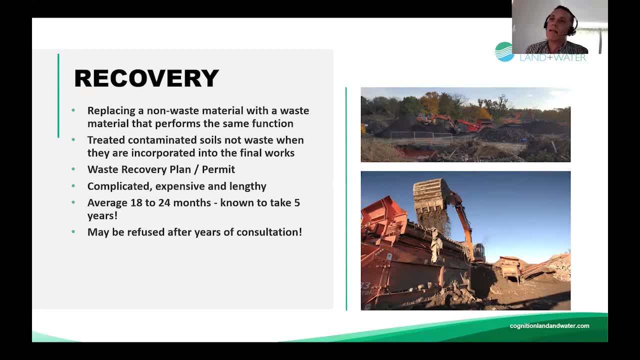 that the process is extremely complicated, expensive and takes forever. to be honest, At the moment the average is 18, a year and a half to two years, but I've known examples that have taken up to five years to get an environmental permit in place, And even after you've been in. 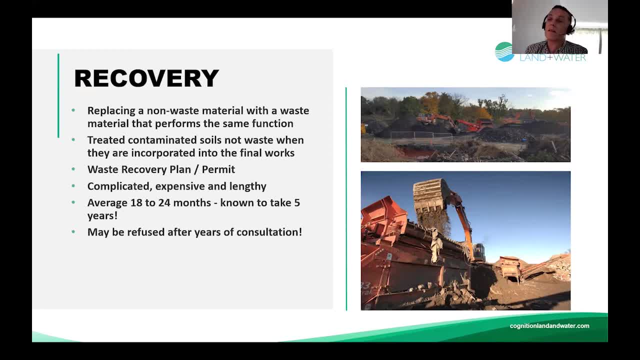 consultation, for in some instances I know an example where the consultation lasted for three years and they just couldn't get it over the line, couldn't agree the details of the waste recovery plan and the environmental permit and it was thrown out And 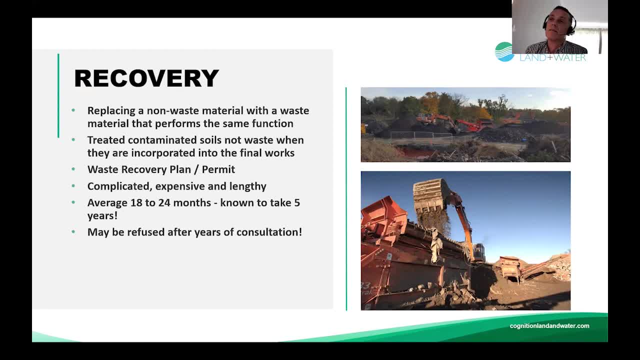 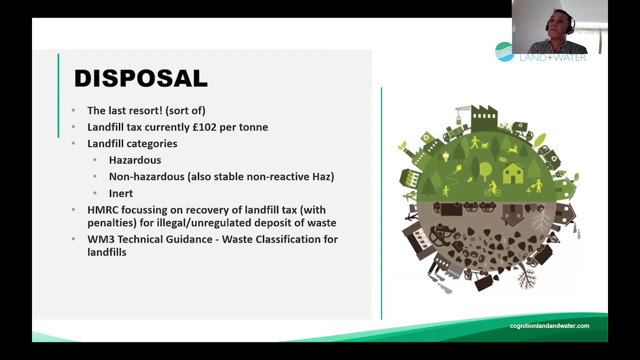 the development didn't go forward. I think that's pretty shocking really, and not the way that we want to move forward in terms of sustainable development. And the last option, as I've said, sort of because really at the moment, because 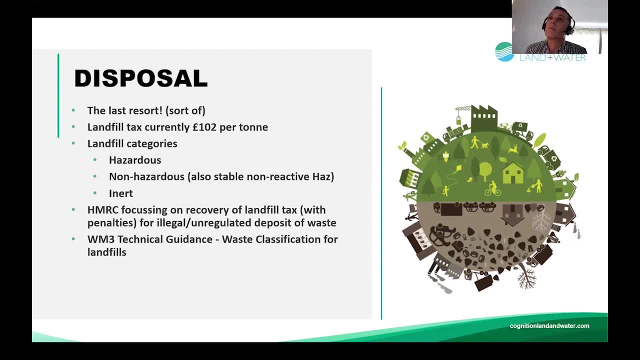 getting an environmental permit or a recovery permit is so difficult at the moment we are having to dispose of more soil than we want to If the program of a development requires it. I don't know of any project that can wait for two to three years to get an environmental permit in place. Landfill tax on landfills is currently. 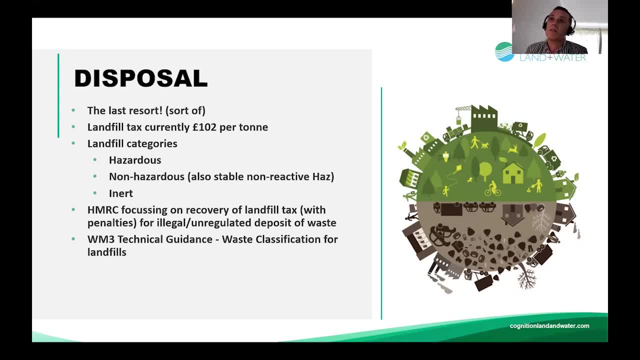 102 pounds a ton, which, as you can imagine, is racked up very quickly. There are several different categories of landfill- hazardous, non-hazardous and inert- And it is important to know that. I mentioned earlier on that you may unwittingly be. 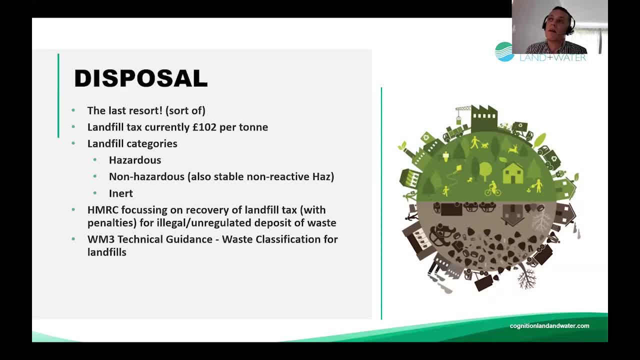 carrying out a waste activity on your site if you don't have the correct process and paperwork in place. HMRC have become very focused on this because landfill tax is so high. It's a big revenue stream for HMRC, So they're going out and looking for sites. 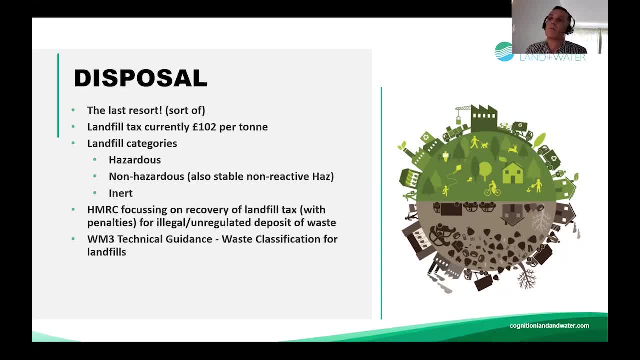 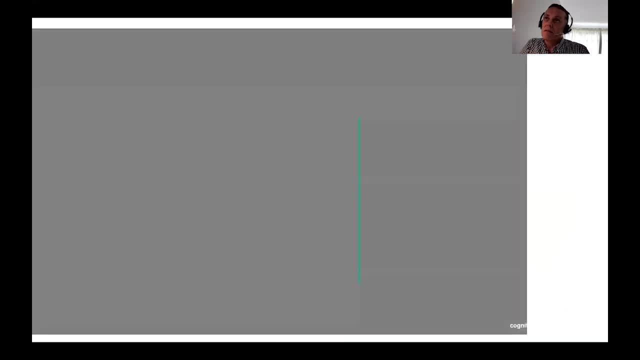 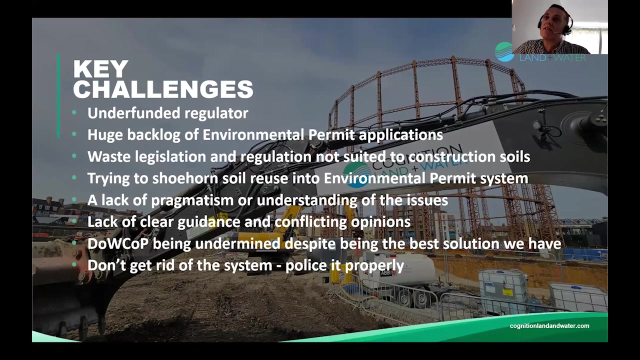 that have illegally deposited waste and haven't regulated correctly. So those are the ways that you going down through the waste hierarchy that you can actually regulate waste. But, as I said and I intimated a couple of times, there are some key challenges for us as an industry. 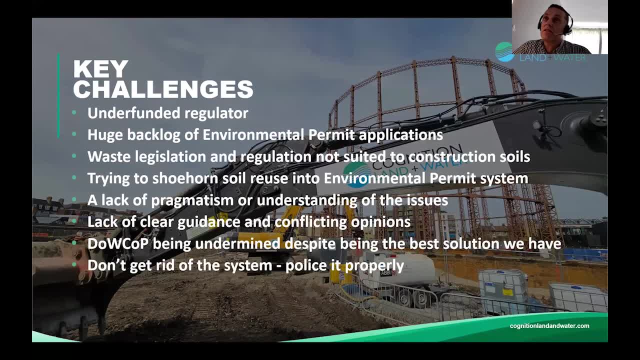 And I think probably one of the bigger ones, which is not the fault of the Environment Agency, is that they're underfunded, hugely underfunded, And you can blame your government and DEFRA for that and maybe think about that tomorrow when you're voting, if that's not too contentious. 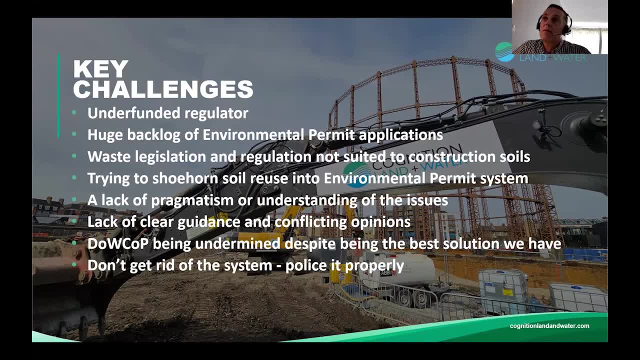 And in the Environment Agency there is a huge backlog of environment permit applications which really is stymieing progress on this issue. Waste legislation and regulation I don't think is suited to construction soils. It's really set up for your typical domestic landfill or an industrial process. 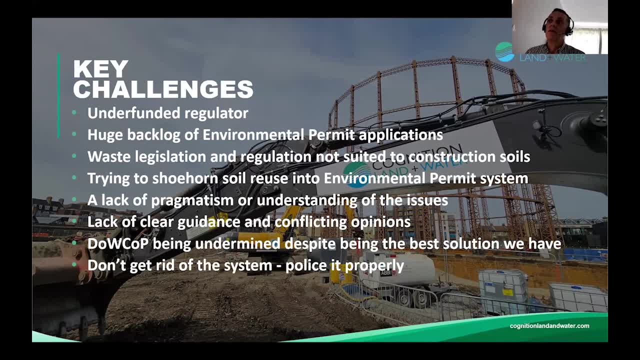 I think we need a different system for construction soils. As I said, there, we're trying to shoehorn soil reuse into the environmental permit system and it really isn't working at the moment. There seems to be a lack of the environment permit system. There seems to be a. 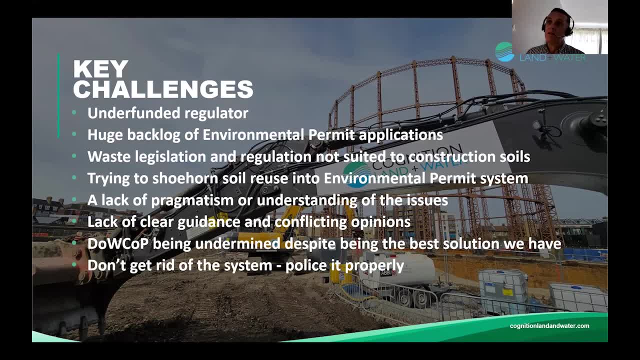 lack of pragmatism and understanding of the issues in some quarters of the Environment Agency and in the regulators and a lack of clear guidance And there are conflicting opinions. We've been waiting for, I think, two to three years now for version three of DATCOP and some 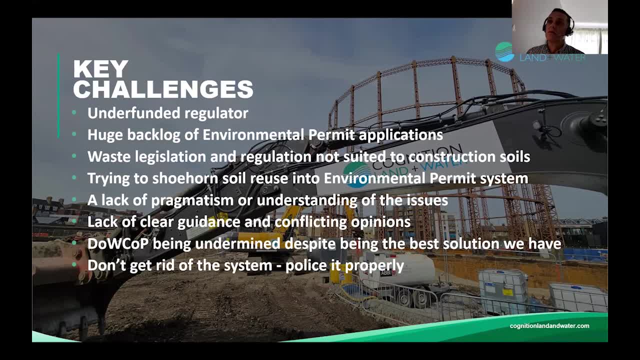 internal guidance from the Environment Agency, and it's just not forthcoming. So we're in the dark really at the moment, And I think recently, DATCOP is being undermined. It's hugely useful too In the industry, And I think it's the best solution, the best tool that we have. But 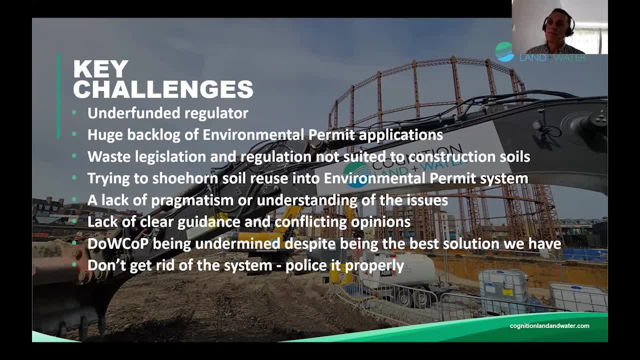 there is resistance to using it in some quarters. Some will say that the system- DATCOP- has not been used properly in the past or has been abused. That may be the case- Our industry isn't perfect- But I don't think you should throw. 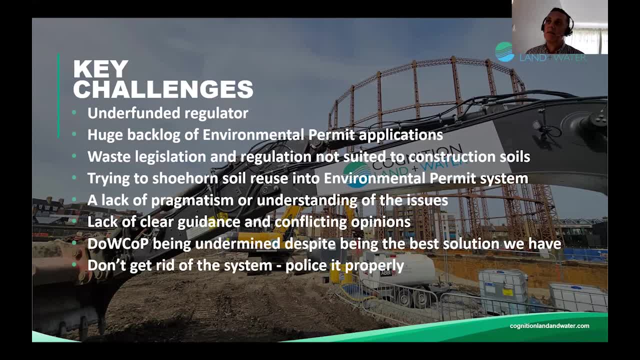 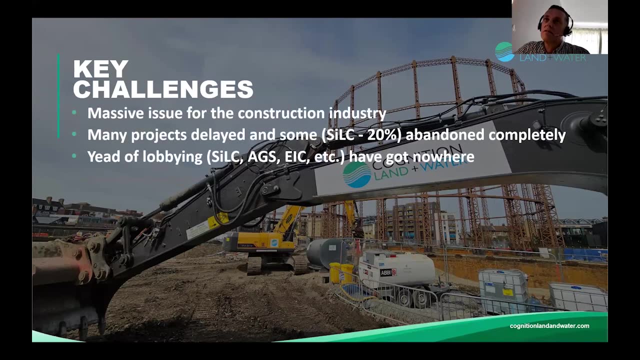 a baby with a bathwater. You don't get rid of the system, Just regulate it, Police it properly, Convict people, Take people to task if they're not doing it properly. As I said, it's a massive issue for our industry. Many projects are delayed and 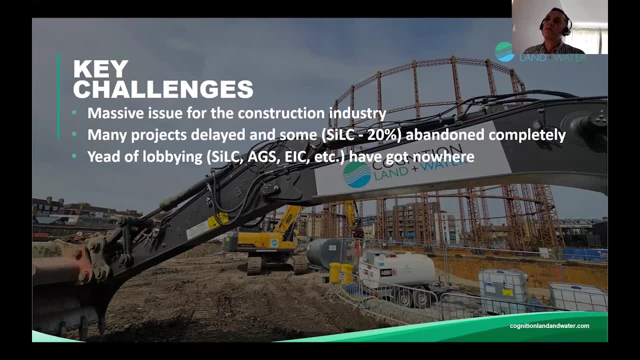 CILC, which is Specialist in Land Condition Organization. they did a survey recently and got a response to 20% of the responses And it's been really helpful. So we're in the middle of the process, We're looking to see what happens And I think a lot of our projects have been abandoned. 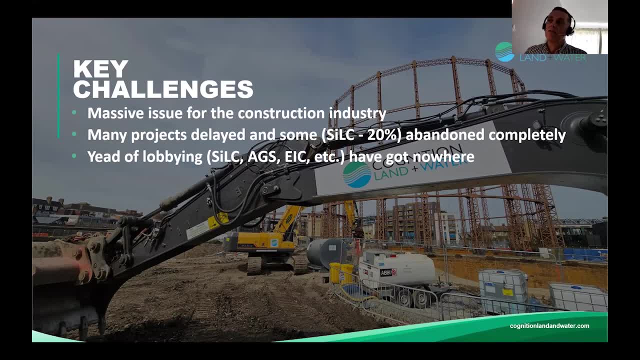 completely recently And I know of three large residential developments with about 750 or so units that just haven't gone forward because they can't wait around for the permits and the funding has been lost. We've been lobbying- That should be years of lobbying- for CILC, AGS, ERC, and we 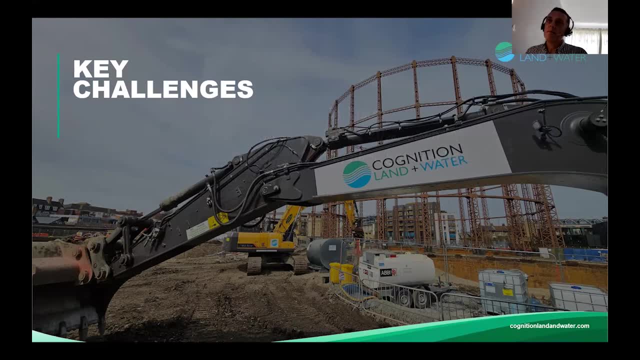 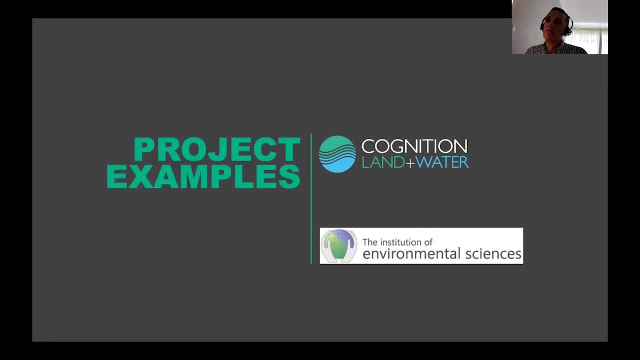 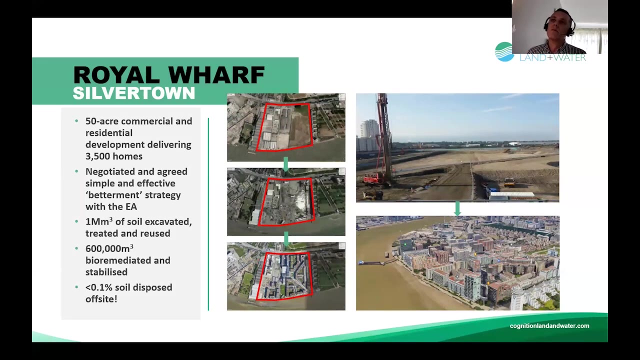 don't seem to be getting anywhere at the moment. I'll skip past that because I'm running out of time a little bit, but, um, i've got a few quick project examples, um that, uh, i'd like to show how this can work well, uh, if it's managed properly and if the if the correct process are used. uh, this is a site. 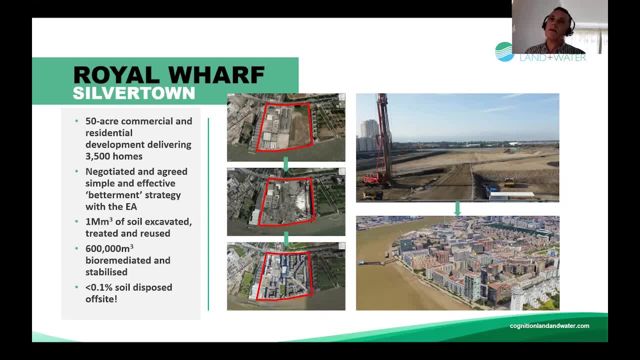 that we worked on for six odd years um a 50 acre former commercial- uh, or sorry, industrial uh- site that was redeveloped for three and a half thousand homes. um, we negotiated and agreed um a remediation strategy with the environment agency and in the end we agreed that, uh uh, it allowed us. 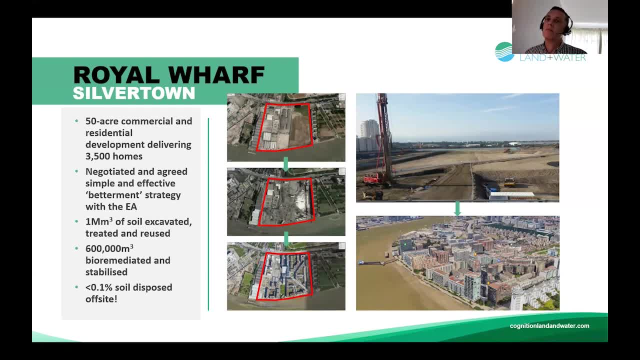 to uh, excavate trees and reuse a million cubic meters of soil on the site. from this um, from this formerly content, formerly contaminated um piece of land, 600 000 cubic meters were by remediated, by mediators, or stabilized, and i think, tellingly, the the last figure there- no point, less than 0.1 percent of soil. 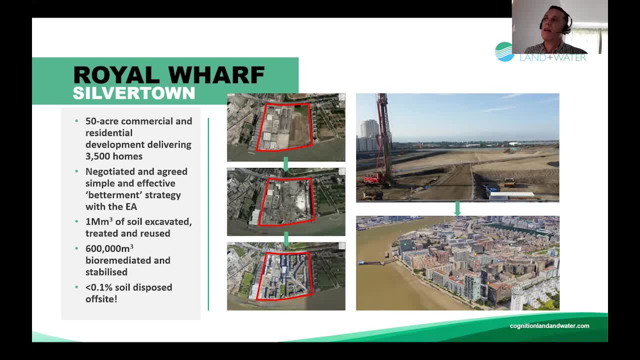 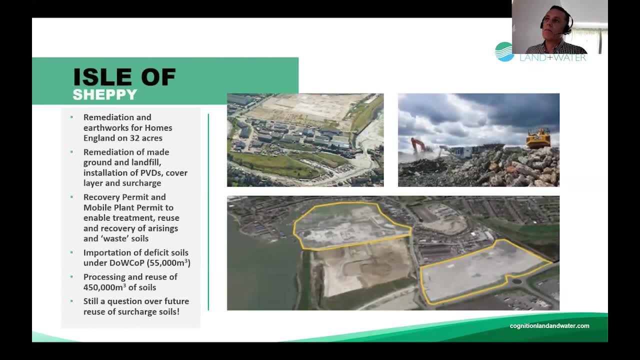 was disposed of off-site. so basically we reused everything on this site within the works. uh, a similar project, this one was for homes, england, on the island of sheppy, a 32 acre site, a former chemical works- uh, a steel rolling mill. and again this was remediation of may ground, a small area of landfill. it also 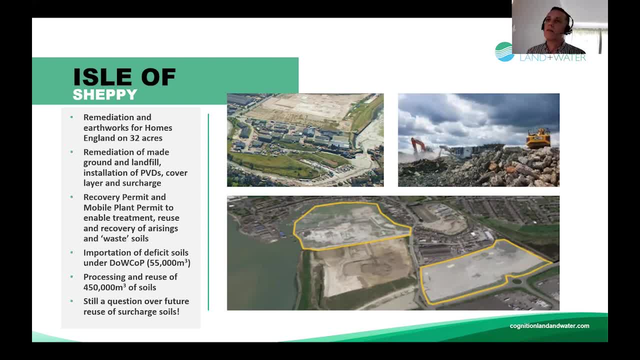 had poor ground conditions so we had to improve the ground as well, using pre-fabricated vertical drains and and surcharging. but all of this work was done under a mobile plant permit. but we also had a recovery perm. we did get an environmental uh recovery permit on this particular one, um for. 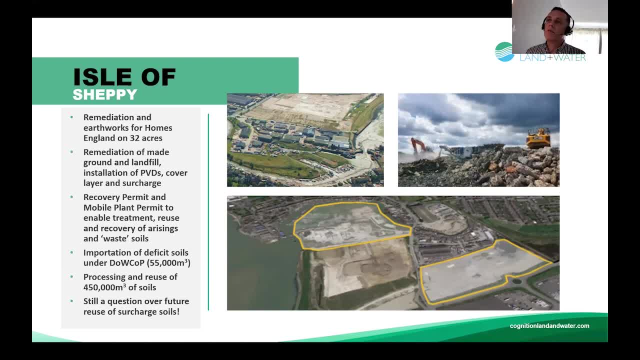 the processing and reusing of these materials. but we were fortunate because there was already an environmental permit in place. but we were fortunate because there was already an environmental permit in on an adjacent site. So all we had to do was to change the boundary and add in a few more. 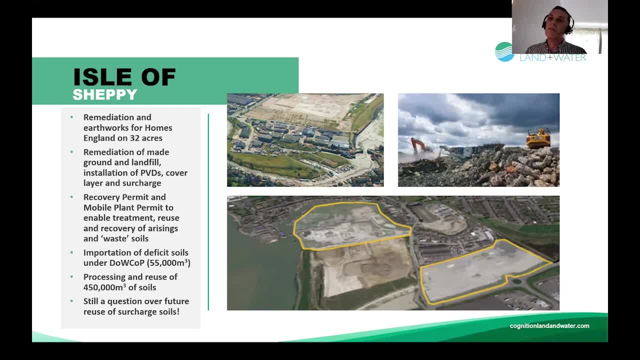 specific details about the work that we were doing on our site, But even that took us eight months just to get that amendment to the environmental permit. In the end we imported just over 50,000 cubic meters of soils for the surcharge and the cover system and that was done. 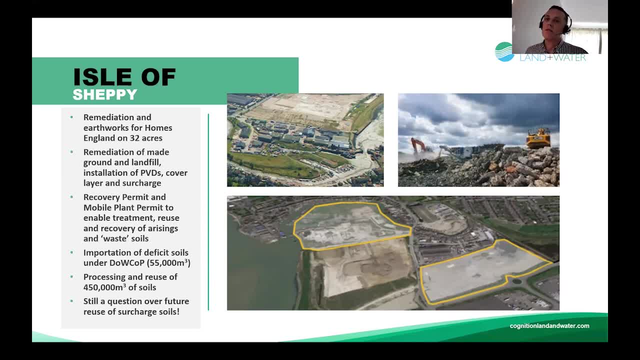 under Dowcop and overall on these two sites we processed and reused for almost half a million cubic meters of soil. But interestingly there is surcharge on the site but there's still a question over the reuse of that surcharge material. This is a clean, naturally occurring soil that was brought 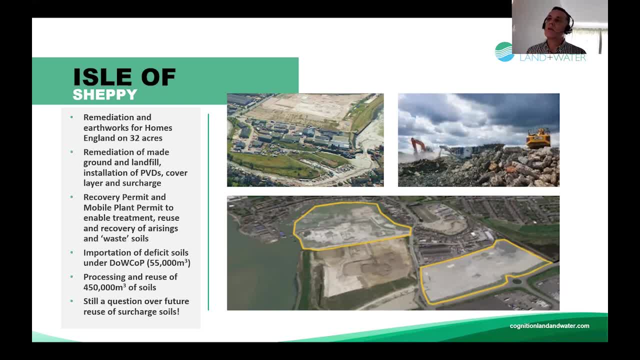 onto the site under Dowcop. but there's a question now as to whether that is a waste and what happens to that material. Can it be reused on the site? Does the does it have to? does the environmental permit have to be extended again to allow that to be reused, or can it be done on the? 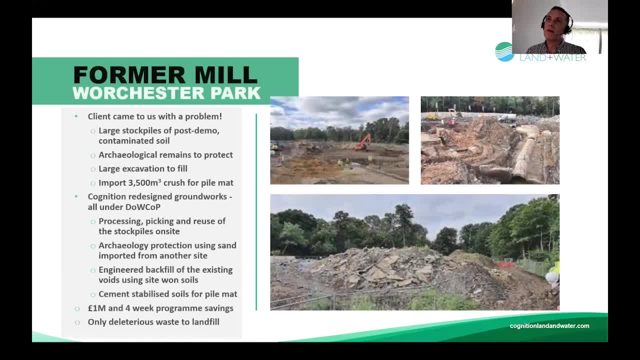 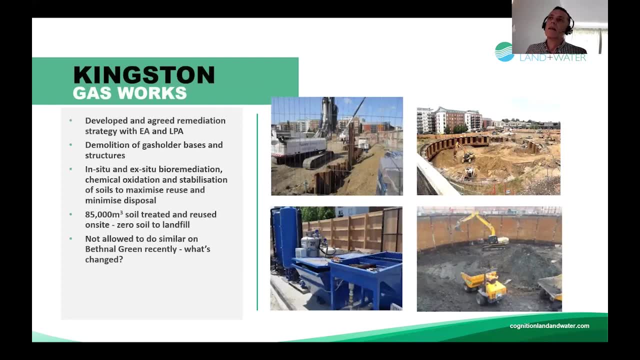 site under Dowcop. We haven't got to the bottom of that one yet. I'll skip past that one because I am conscious of time. and then there's the last one, which is a gas works in Kingston in London. This is one that we did a few years ago. We developed and agreed the remediation strategy. 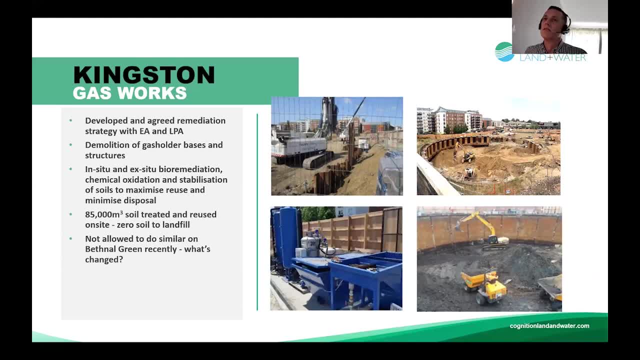 with the Environment Agency and the local authority. This involved the demolition of the gas holder bases and the structures, but it was contaminated. as you might imagine. We used bioremediation, chemical oxidation, stabilization of soils. All of those basically threw everything at it to maximize the reuse of soil and minimize disposal. 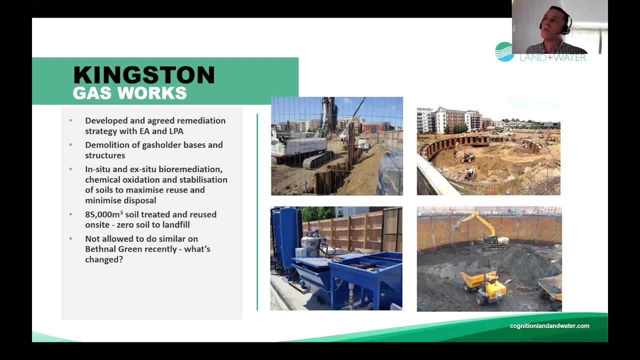 In the end, we treated 85 000 cubic meters and zero soil went to landfill. Everything was reused within the works. However, we're working on another site more recently at Bethel Green, and on that site we're not allowed to do exactly the same process. 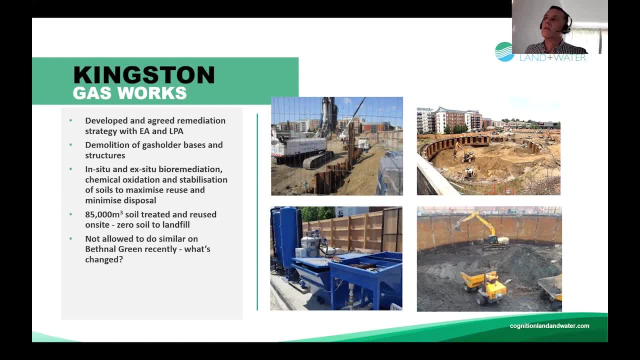 uh, any contamination of soil, any contaminated soil that's above the agreed reuse criteria on that site have to be disposed of off-site. they can't be treated, they can't be reused within the works. now, to me, i think that's that's well this way. it's madness, i think it's. um, we really. 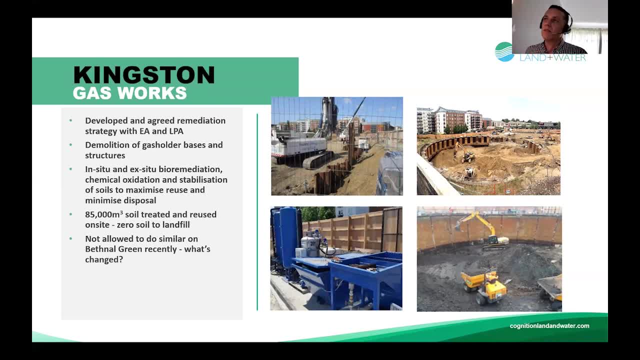 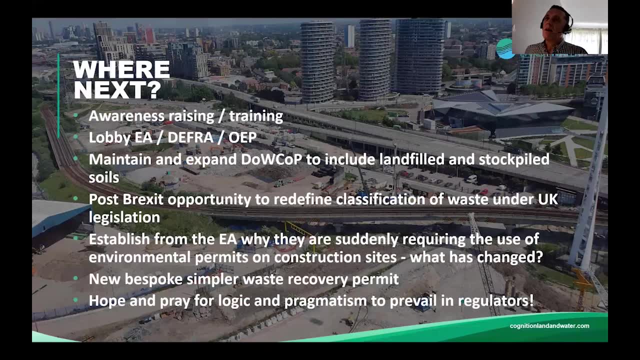 should be treating those soils and reusing within, reusing them within the, within the project. so where next last couple of slides? um, i think it's really important that we raise awareness and that's why i'm talking today, putting my neck on uh out a little bit, really. uh, i've been quite 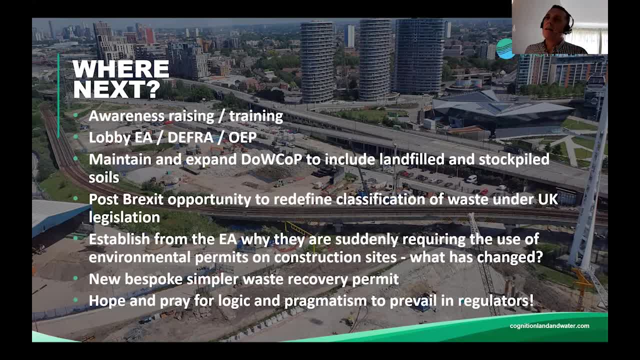 um, but uh, maybe a little bit controversial. um, we need to raise awareness, but also um train people and understand um how to use these processes properly. i think we need to lobby the environment agency, defra, even the new office for environmental protection- who are essentially the police for the environmental agencies, so we're looking to talk to them as well. 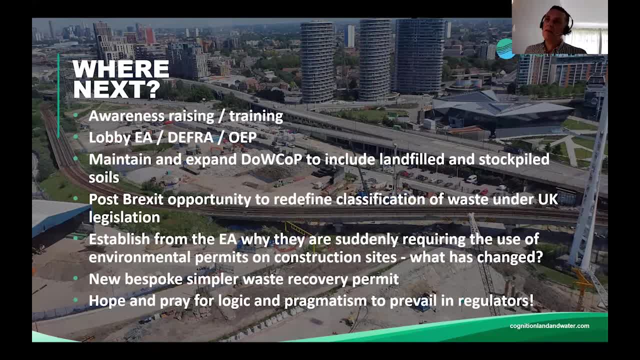 um, i think we certainly need to maintain dow cop, but i also think there's an opportunity to expand us to to specifically allow for um reuse of landfilled materials if they're suitable for use. i'm not talking about digging up domestic landfills and talking about 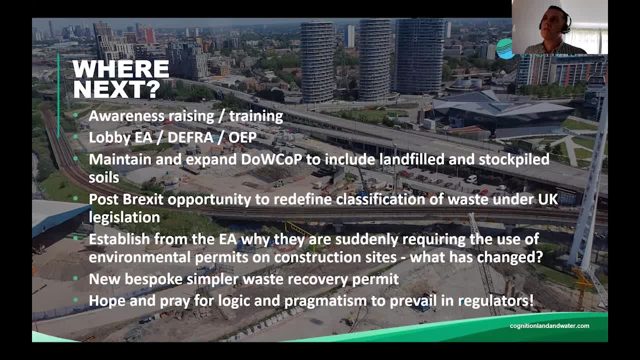 uh sites that are suitable for for use with large quantities of recoverable soils and stockpiles as well. that's a. that's an issue that, um, that crops up quite a bit. is there a? i'm no fan of brexit, i can tell you, but um, is there a post-brexit opportunity to? 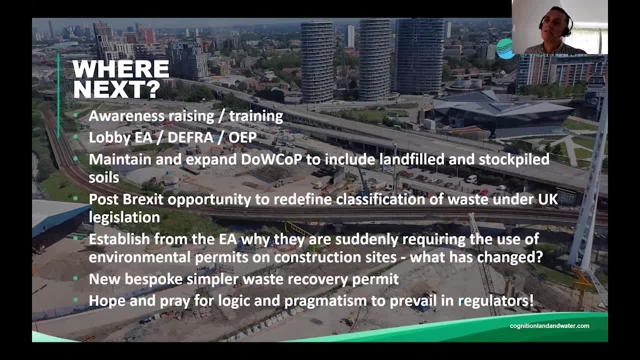 redefine the classification of waste under uk legislation, something that we're looking at um and really to understand us from the environment agency, why there? there? there is this change of heart, i suppose in requiring the use of environmental permits on construction site. what has changed? maybe we could look at doing a, a formulating a new, bespoke, simpler waste recovery permit. 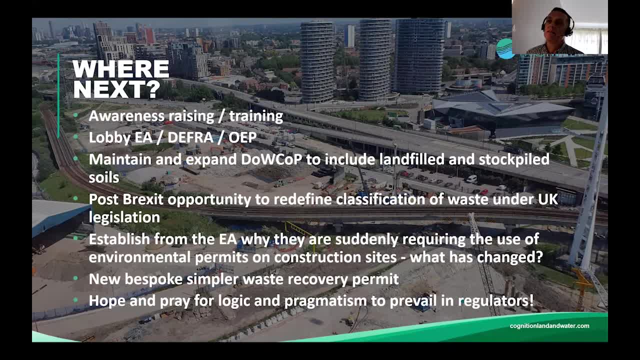 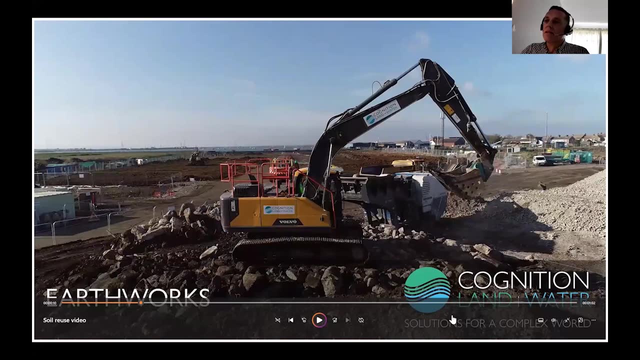 which that doesn't take two to three years to to get in place and, being the eternal optimist, i hope and pray for logic and pragmatism to prevail both in the regulators, but also in the industry as well ourselves. i have a very quick video just to play um. hopefully this will work. 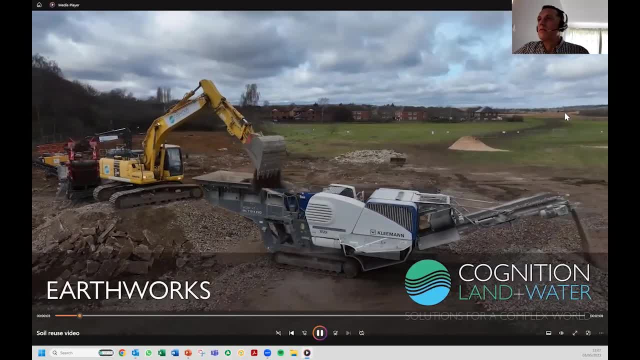 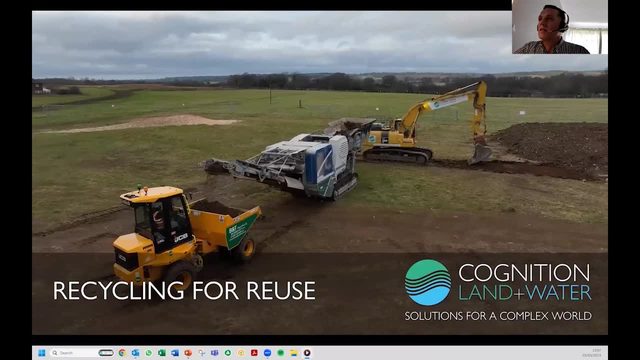 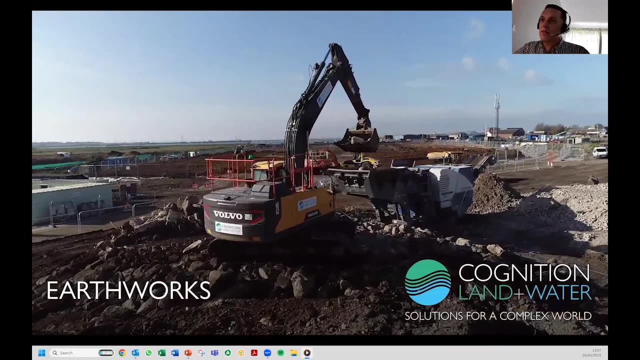 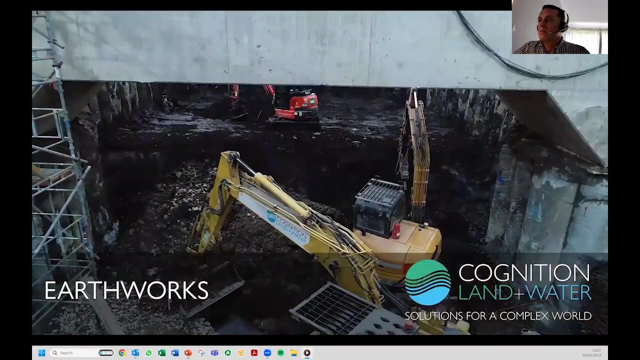 Yeah, so these are just some examples of how we carry out reuse, processing, recycling of soils on various sites using lots of different technologies, remediation technologies, just some simple technologies as well, such as crushing demolition horizons to produce 6F2.. 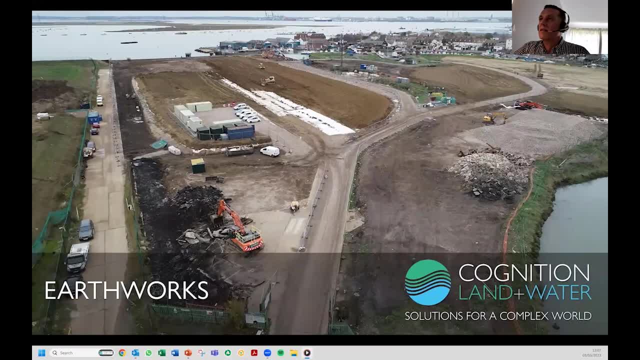 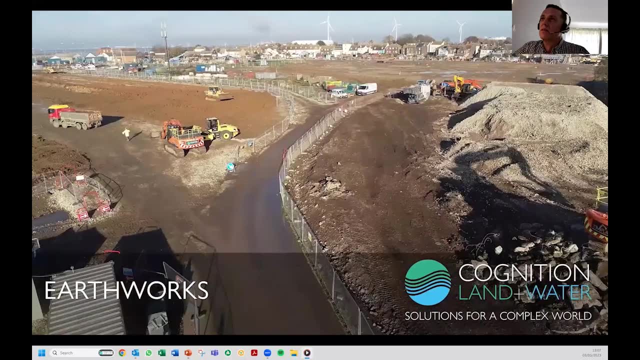 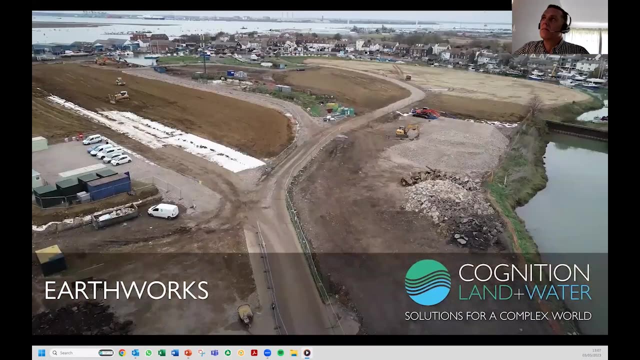 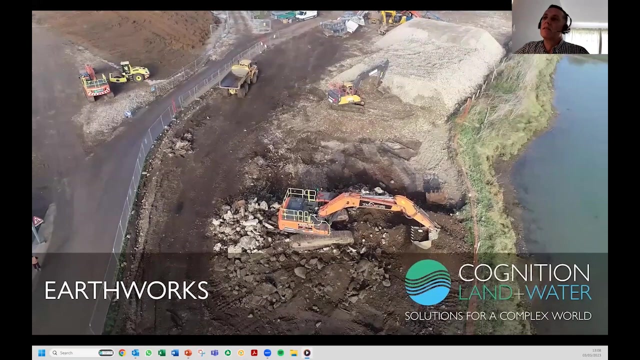 That last one was an excavation of a launch chamber for a TVM in Silvertown where we reused all the excavation in the enabling works. We processed and treated and reused the materials on site under mobile plan permit and under DATCOP. This one is the site in Sheppy that I was telling you about. You can see this processing of 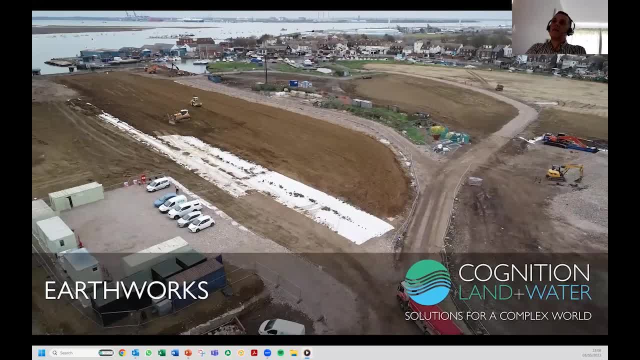 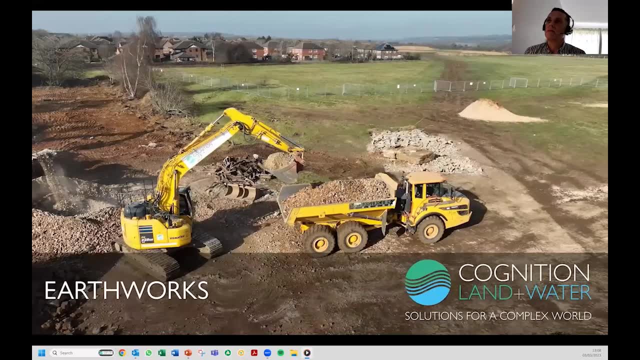 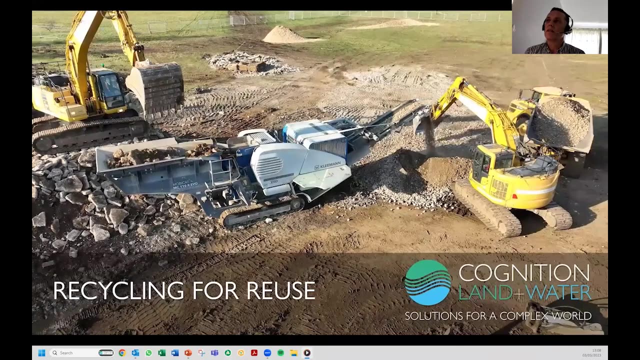 materials, but then also that white geotextile there. you know that's on top. that is the cover system, um to protect uh future users of the site. all of that material was um, was brought in under dad, cop and uh from other sites and that's pretty much. 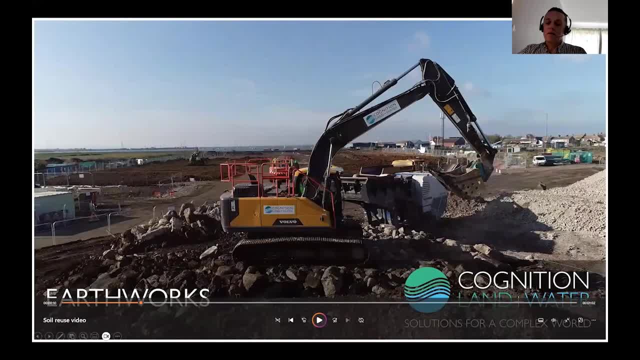 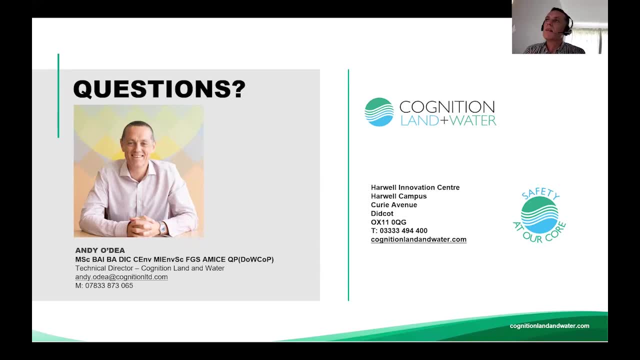 it. um, yeah, lots of things to think about. i'm more than happy to take questions. i haven't seen the questions come through. um, i i'm happy to answer any of those, but also you have my details there. if people want to get in touch with me to talk about this, then i'm more than happy to second. 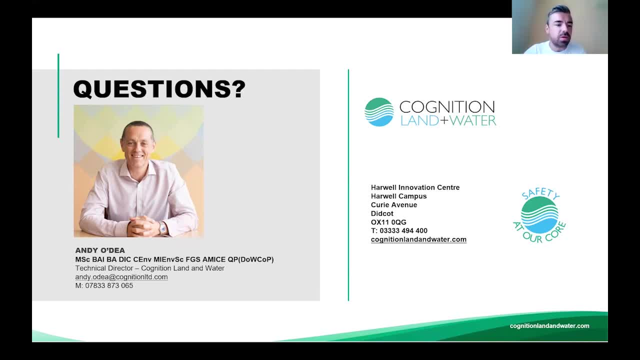 questions. fantastic. thank you, andy. um, it's always great to see um the different examples and when you're talking about these challenges and the different methods. and we do have a couple of questions and before we get started, i'll ask one: um, just why do you think there's a resistance? 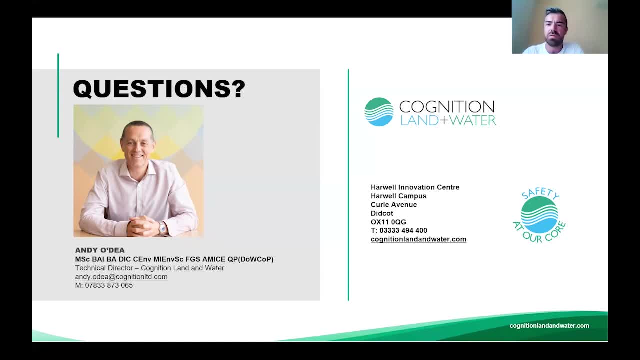 um, to use the um do cop. i really don't understand, because i think it is such. if since 2008, it has been such a really beneficial tool to our, to our industry, i i think maybe people, uh in the regulars, have looked at it again, maybe the legal people have looked at it again and decided that, uh, there are certain 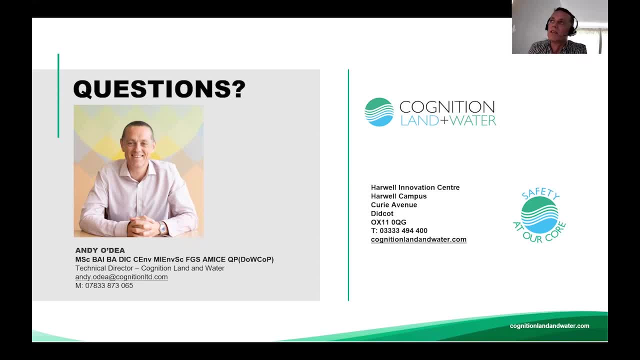 instances where it doesn't exactly fit with the- uh, the waste legislation. and i do understand that there's this sort of um conflict between some people in the agency who really want to see it succeed and move forward and others who say that you absolutely have to comply with um, with legislation. uh, i agree we have to comply with the legislation, but if the 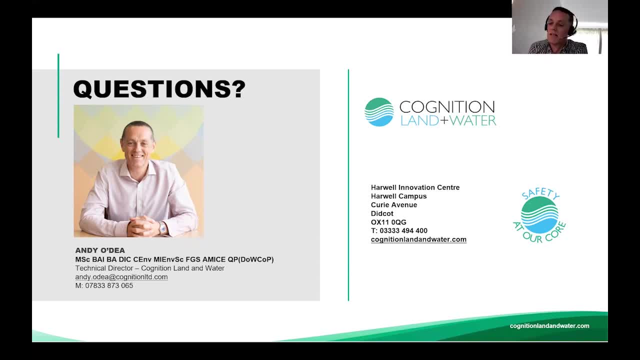 legislation is wrong- clearly it's wrong in some instances- then we need to do something to get get over this, this impasse. it's succeeded before it's um, like the one of the slides that i skipped past there quickly was the employment agency and i said that any landfill waste is it definitely. 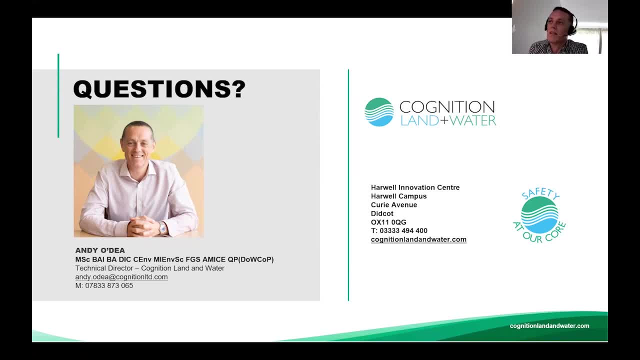 cannot come under danko. but when backup was launched originally, there were case studies on the clare website showing exactly that: re um reuse, regeneration, processing of landfill soils and reusing them within the site- all under tackle. that's no longer allowed at the moment. perfect, thank you. we've got a couple of 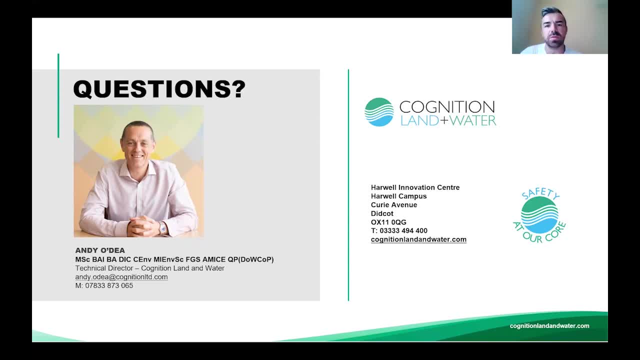 questions on um mmp. so i'll just kind of ask those um. so matthew's saying: hi, andy, thanks very much for an interesting presentation. what are your thoughts on the need to use an mmp under doubt cop for a construction scheme that is on a green field site only? the reason for the mmp is to demonstrate that the material 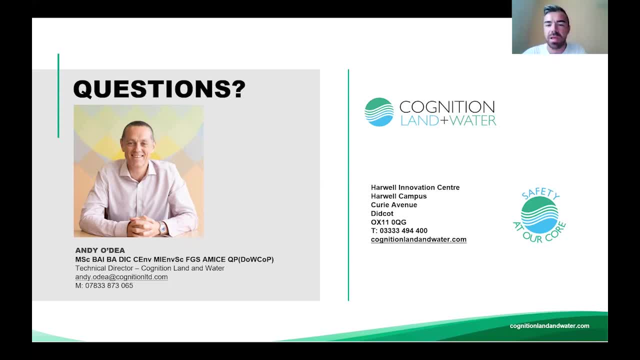 is not a waste and is therefore not subject to waste legislation. legislation, however- wage legislation, sorry. waste legislation states that the uncontaminated soil and the naturally occurring material excavated in the course of construction activities, where it is certain that the material will be used- used for the purposes of construction in its natural state on which it was excavated, is. 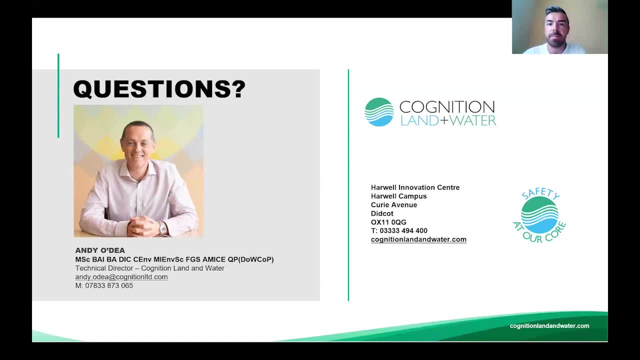 um. so yeah, i think the question there was. um i i yeah, i understand the question. i think i suppose this goes back to my point earlier on that um, a soil doesn't have to be contaminated to be a waste. there are two completely different sets of legislation, um, so waste legislation and 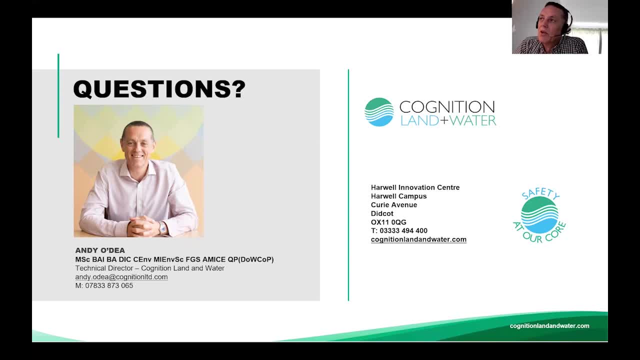 contaminated land legislation um are not the same. so even if a top soil is is excavated, or a natural gravel or non-declarated or something like that, that's absolutely can become a waste if it's not managed properly. So I would say that if material is reused on a 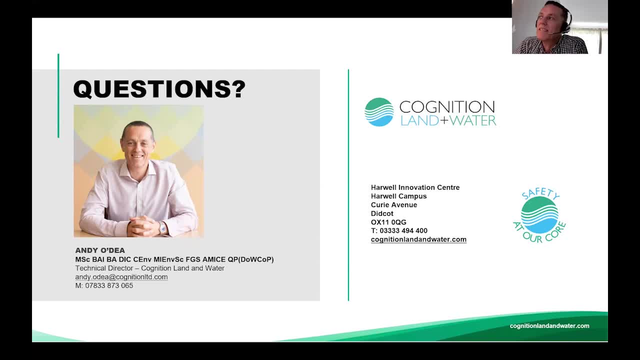 site. the natural material is reused on a site, then you don't necessarily have to use and there is a position statement that says that you're exempt from waste legislation if you reuse natural soils on site. But I would suggest that an MMP is the best way to make sure that you're covered. 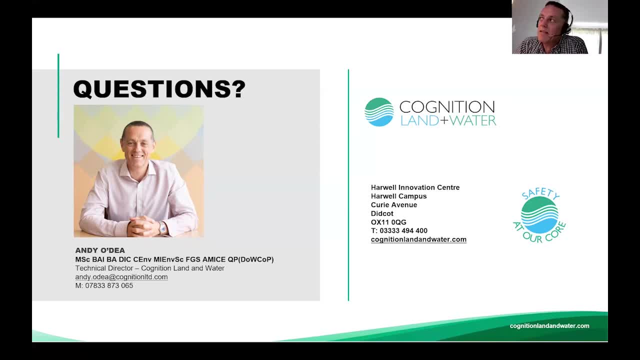 that you have demonstrated to yourself and to the Environment Agency that your operation is not a waste operation, even though the material isn't contaminated. And an MMP is not expensive. The administration fee is £165 for up to 5,000 cube, I think, and then it increases for values after. 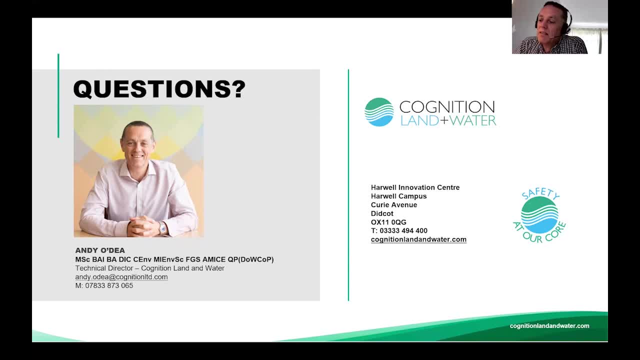 that But and producing an MMP is not an expensive business, especially on a large construction site, So I think it's probably useful to have as a process to make sure that it embraces that what you're doing is not a waste activity. And what changes would you like to see the MMP process and the forthcoming items? 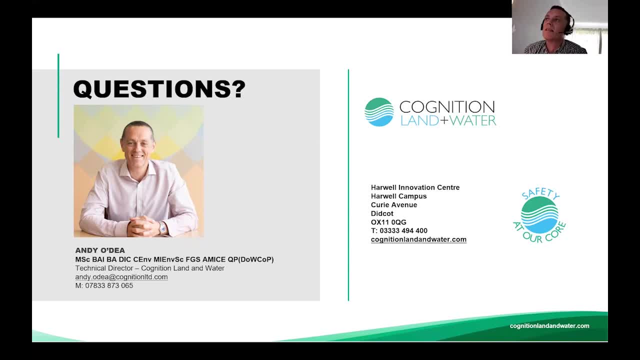 I'd like it to be categorical in saying what is allowed. I'd like it to include landfill soils. I don't see why that shouldn't be. that should be an excluded activity. It was in there before what's changed. Why was that? Why is that being excluded now? Also, as I mentioned, 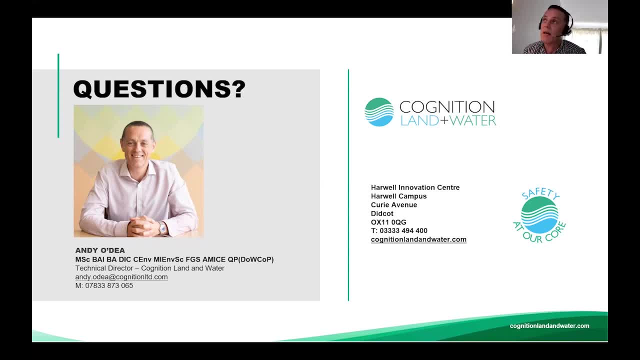 earlier stockpile soils. that is a difficult one, because that has shown that people haven't planned properly, planned for the reuse of other material and have stockpiled soil on the site. you could argue that that if there wasn't an exemption, it wouldn't be a waste activity. So I think it's. 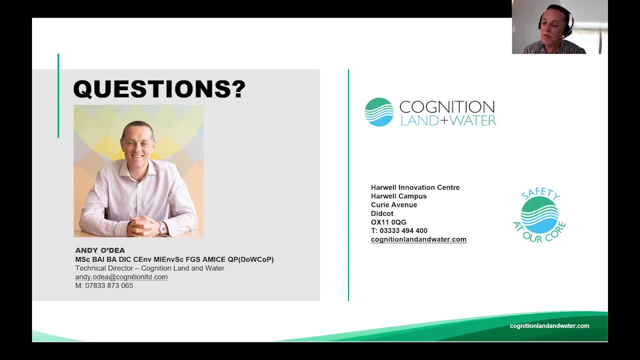 that if there wasn't an exemption in place, and that's or that's been there for more than 12 months, that is a waste And I understand that. But if we can't get an environmental permit for the reuse of that material, then what options do we have? We can't wait for two to three years to. 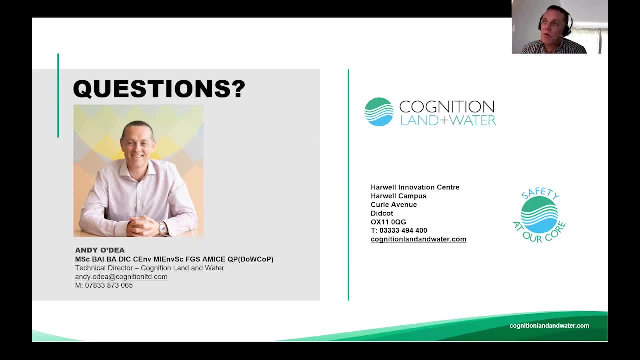 get an environmental permit in place. If we can't use Dowcopp, then there's no option but to send that material to landfill, And that is a disgrace in my mind. We need, we need to find a way through, and I think Dowcopp is probably the best way to do that. 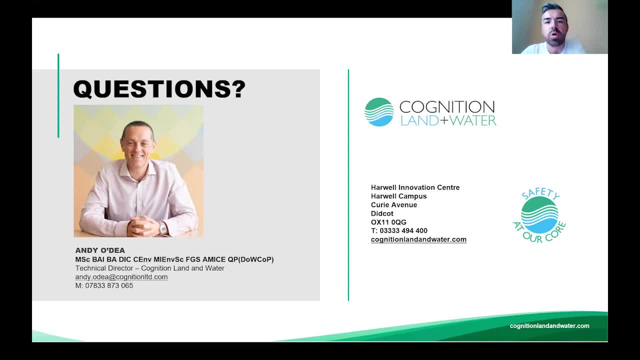 And I think Dowcopp is probably the best way to do that. Kerry is asking what proportion of soil wasted from construction site is defined as contaminated. Oh, that's a difficult one, The definition of contamination. there is no hard and fast definition. 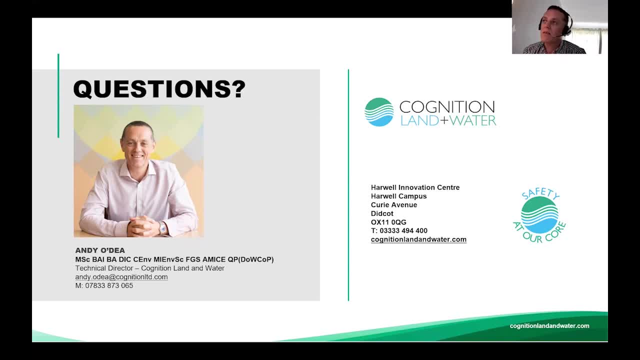 of what a contaminated soil is, because it all depends on the pollutant linkage. So you're going back to your source pathway receptor scenario: If a soil can be contaminated if it's used in one particular situation and not contaminated if it's used in another situation. So, for example, if something has sort of moderate contamination, you 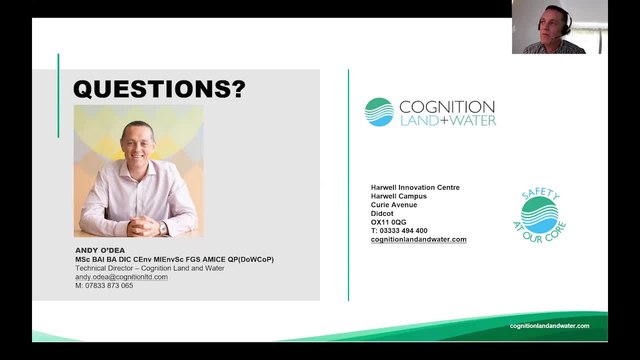 wouldn't use this in a domestic garden, but you may absolutely be able to use this underneath a building or a road or as a fill beneath a cover layer. So there's no hard and fast rule as to say what's contaminated or not, And therefore I can't really give you a proportion. 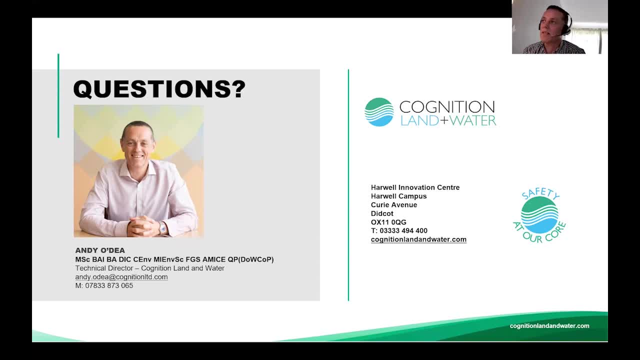 In terms of construction horizons. but on our typical sites the vast majority of material doesn't need remediation. Usually on a typical site we look to excavate out hotspots of contamination, take out the sources, treat those, deal with those separately, and then the vast 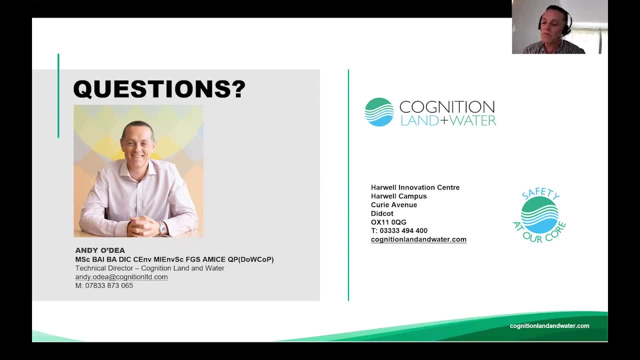 majority of the residual soils, even though they're made ground, are suitable for use within the works. Fantastic thanks, And just to note that we do have quite a few questions, And so we'll just answer a couple of them, Okay. 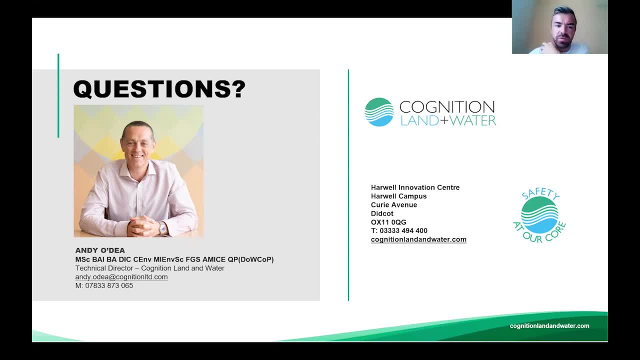 A couple, But Andy has put his contact details on there, So if you want to get in touch, they are on there. I'll just ask this one here from Rebecca: what would be your ideal vision for the way forward for soils reused to be specified and requiring an environmental permit to send material? 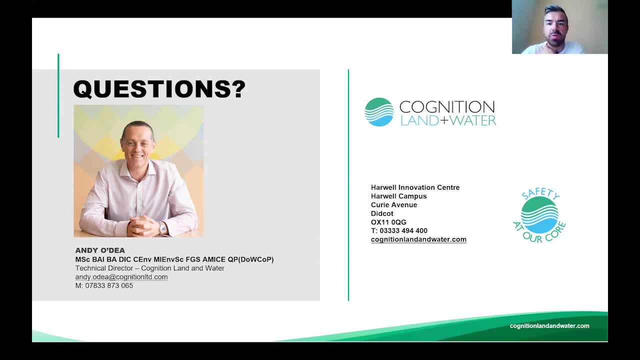 to landfill seems a better way around, assuming appropriate risk assessment and reuse procedures are in place. Not quite sure I understand the question, But yes, so long as risk assessment and has been in place and the soil has been correctly assessed and is suitable for use, then why not be allowed to use it under DADCOP on the site, Environmental permitting. 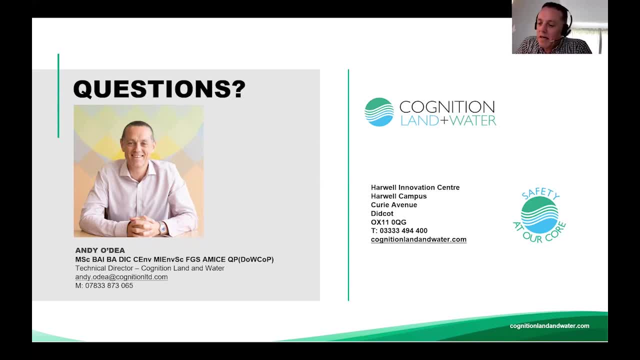 for construction soil is just not working at the moment. You can ask anybody in our industry who is involved in this and they will say the same thing. I don't think environmental permitting is the way forward. I did put in an option there of a simpler environmental permit, if that could. 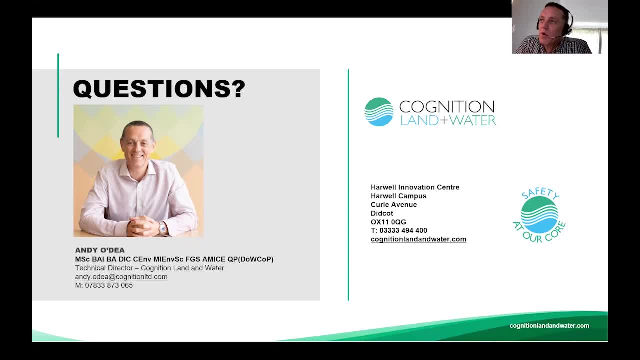 be. if we could have some assurance that that could be dealt with quickly, promptly, within sort of land development timescales, then that might be a way forward Demonstrating that a soil, when it's when it's treated and it's reused on the site, is recovered and is no longer a waste. I think that 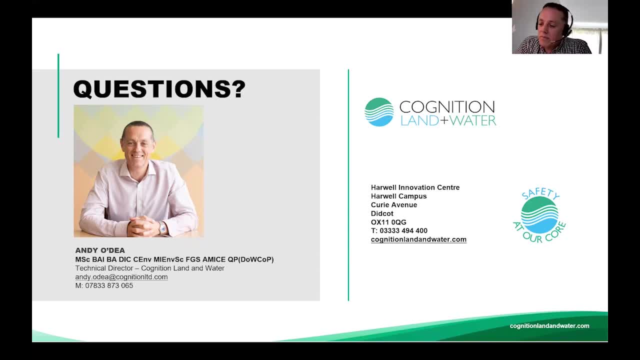 would be an option. But why not include that within the as an option within the DADCOP? I suppose you could have it as a sort of a two pronged approach For different situations. I'm just sort of thinking on the fly here, But yeah, I think I've made it. 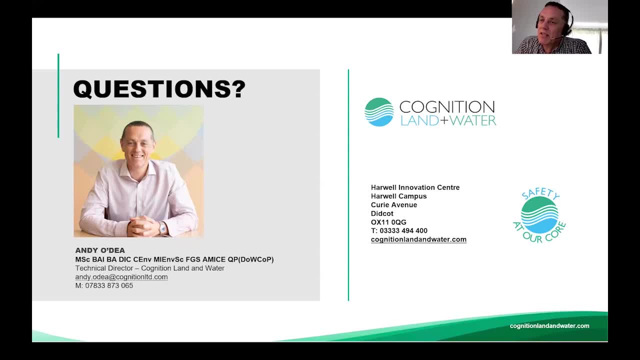 clear that my preference is for DADCOP to be retained and actually expanded, rather than being limited, as it seems to be the way we're going. We have two questions that we'll finish on just around QP. So Zoe's asking: is it still worth considering being trained as a QP now? And the 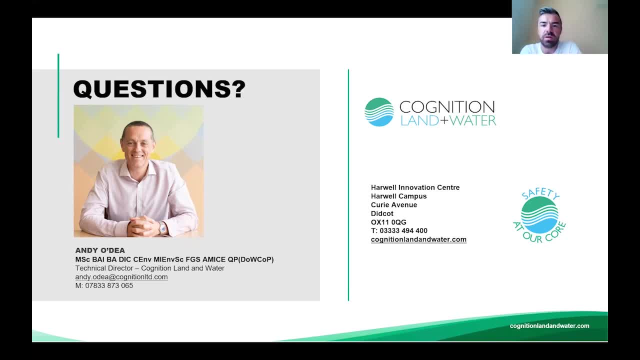 other question is: many would suggest that a QP who works for the company undertaking a project is not truly independent or there's always a more direct financial incentive. Do you think having a standard fee and requirement to be independent from the project company would give more confidence in the regulation of these sites? 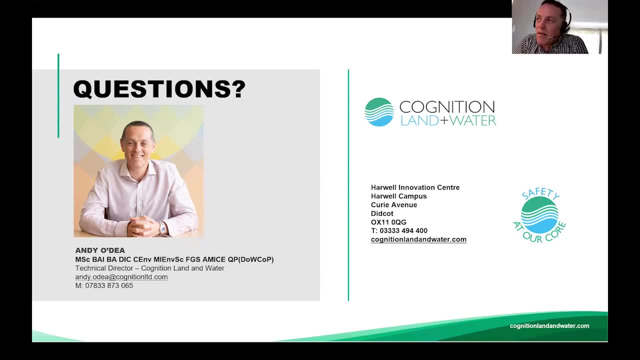 So the first one: yes, absolutely I think we need more QPs. I think it's an excellent system. The training course is really interesting and really good. I know the people who do the trainers they are, who are trainers at Clare. 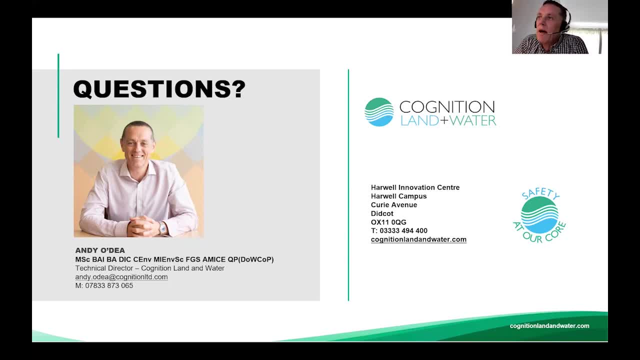 They're very knowledgeable in their trade And even if you don't QP lots of MMPs in a year, I think still as an exercise to allow you to understand waste legislation, waste regulation and the DADCOP process absolutely, I think that I would suggest that you go through that. 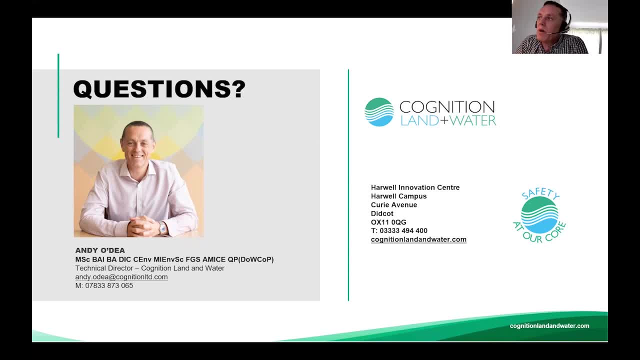 The other one whether a QP should be independent from the company and not just the project. if it did, I don't think it's necessary, personally, because I've QPed lots of. I actually don't QP for projects at Cognition because we have somebody that does it for us. 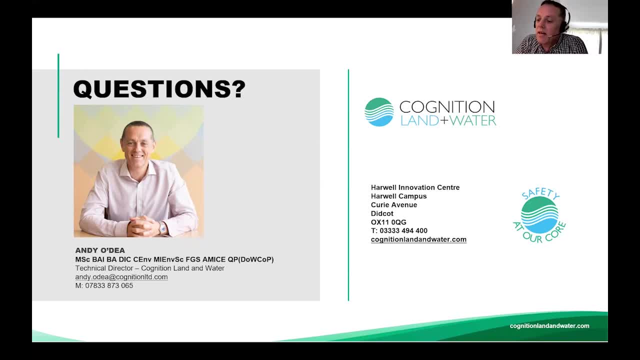 because invariably I'm as the technical director there. I'm involved in the project so I can't QP them as an independent. But in my previous work in a large consultancy I did lots of QPing for projects that I had absolutely no involvement in at all. I had no 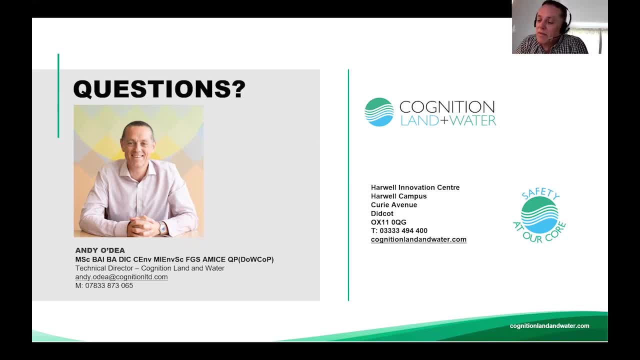 financial incentive or there was no benefit in me taking a slanted view, I suppose, in terms of my review of the MMP. However, if it did give the Environment Agency or the regulators additional confidence that the DADCOP process was being followed strictly, then absolutely. If that was. 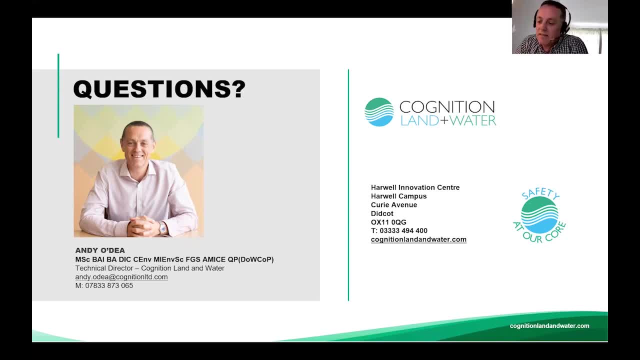 included as a requirement that it was outside of the company, then yes, definitely, But only if there's a benefit to doing that And a standard fee. yes, that could be done as well, but you just need to be a bit careful. Some projects are more complicated than others. A two-house development. 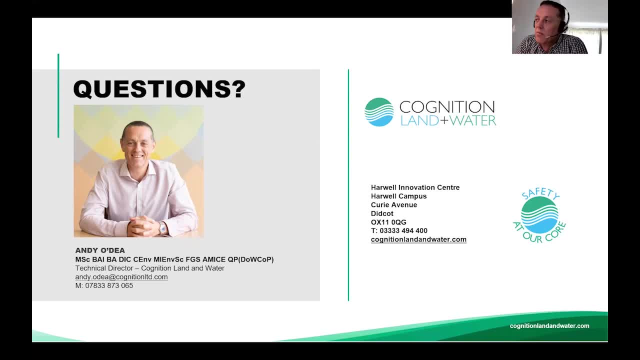 being the QP on a two-house development is a much simpler and easier process than a three and a half thousand unit development, So there possibly may need to be a scale of fees there. Fantastic, thank you. Like I say, I am aware that there's a few more questions that we haven't. 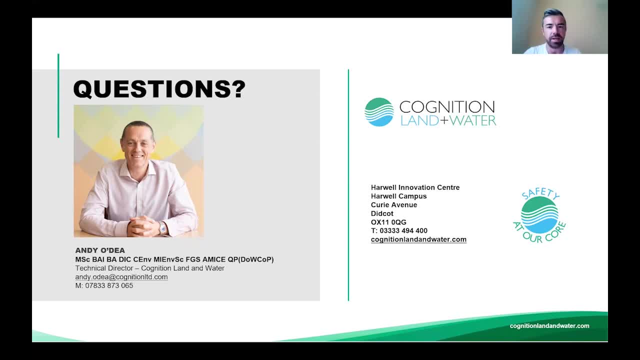 had time for, So Andy's contact details are there if you would like to contact Andy directly, And that's it from us today. Thank you for logging on. I hope you find it beneficial and informative.